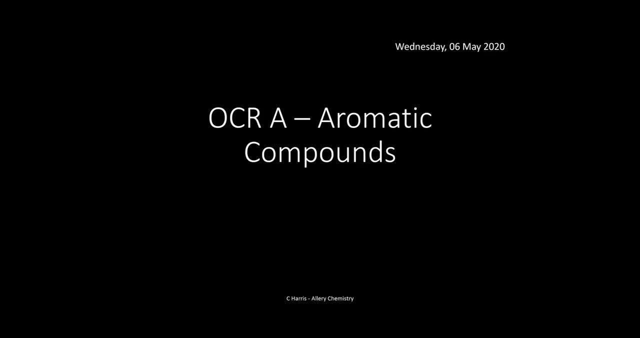 full range of videos for all OCRA year one and year two, and all other major exam boards as well, that are specifically designed for these, for each of their specifications, So they're tailored to that. They're all completely free to use, but all I ask is you please subscribe. 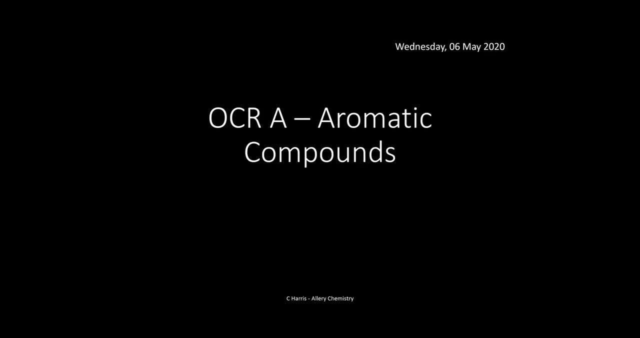 to the channel to show your support, And if you click on the subscribe button, either at the bottom of the video or you can see there's cards at the end as well where you can click on it and subscribe or even just go onto the onto the channel as normal. So. 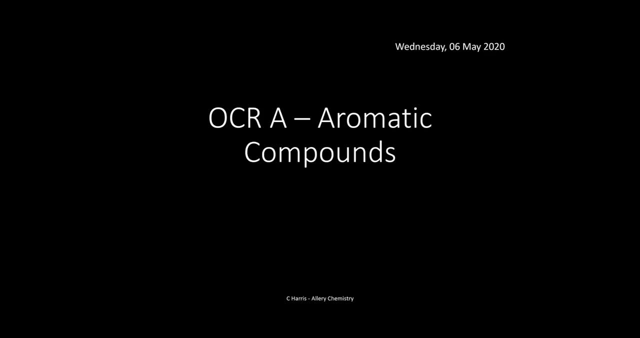 yeah, they're all for free there. but if you want your own private copy of these slides here, they are available to purchase. If you just click on the link in the description box, then you'll be able to get access to them, But the video is obviously completely. 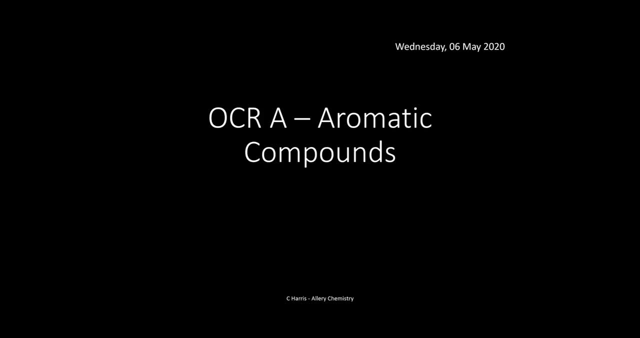 free and all available on the on on Aloe Chemistry. So this video is designed to go through the content. Like I say, it is important to actually go through exam technique as well, because it's one thing, knowing the content it's another. 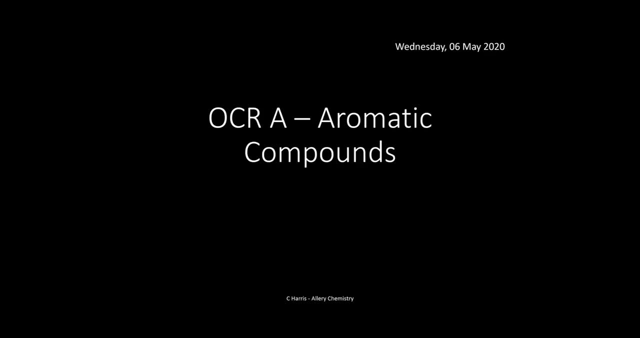 thing: actually putting it into place and and putting it and answering an exam question. Exam technique is just as important. So please, please, practice your exam technique And I have done some videos And if you have a look on Aloe Chemistry where I've gone through, 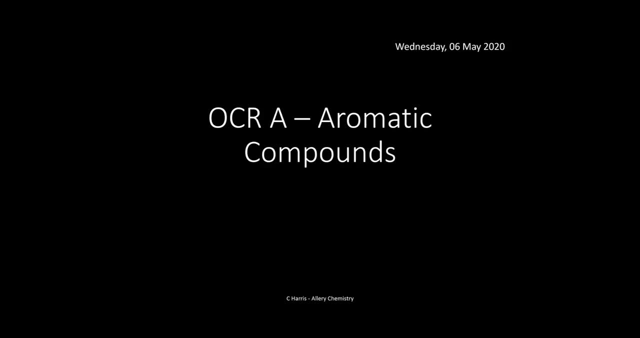 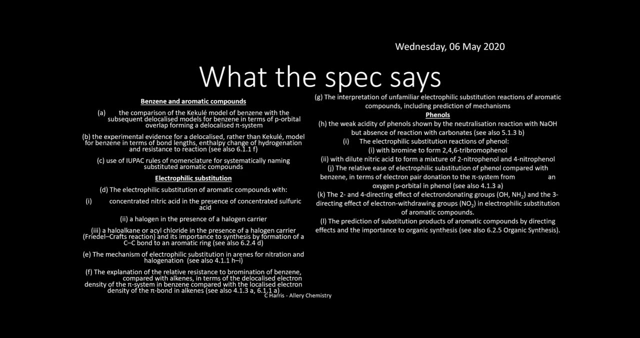 some past paper questions that go through that So you can see. you can see for yourself on there as well. Okay, So let's make a start. So, like I say, this is dedicated to the OCR specification And so it goes through a content such as benzene electrophilic substitution. 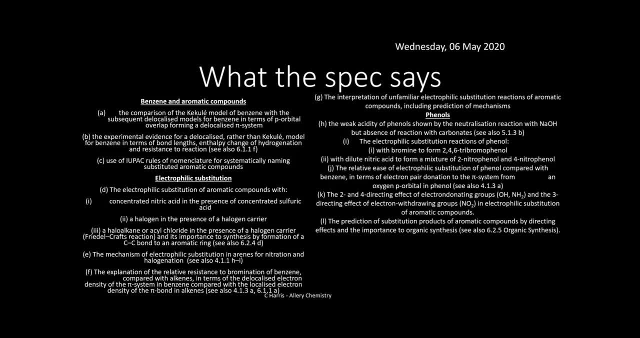 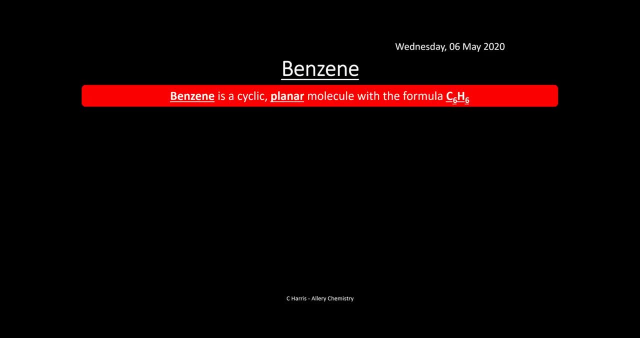 So these are the reactions that happen with benzene and phenols. It's all aromatics, So it's already starting to smell nice already, Right? So let's look at benzene first. So a lot of the topics are going to be on benzene, of course, So we better see what it's about. 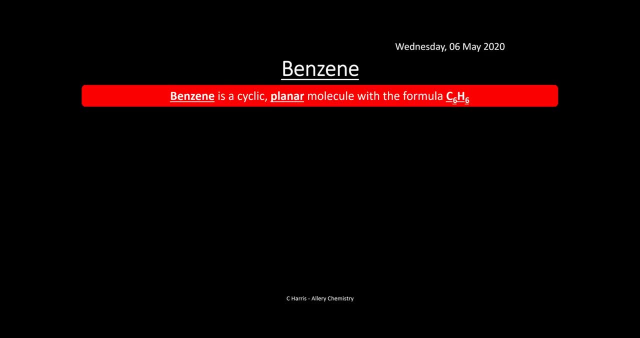 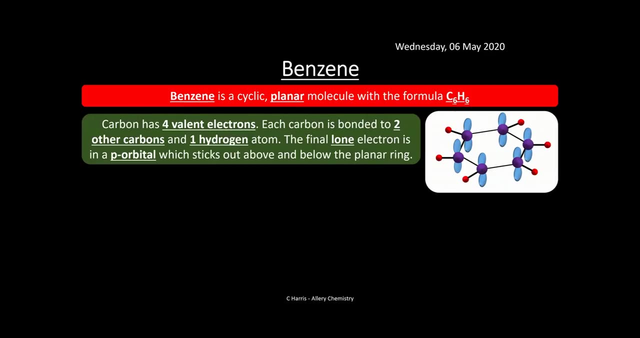 Shall we So? benzene is cyclic, It's a planar molecule, So it's flat and it has a formula of C6H6.. So carbon normally has four valence electrons and each of them, carbons, is bonded to two other carbons in a benzene ring. And you can see on here. you can see, you've got. 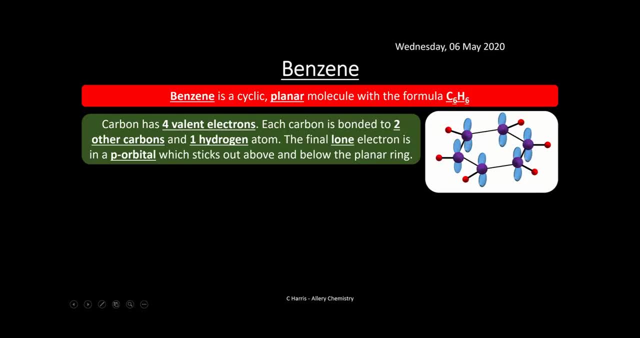 the bonds here, which each, obviously each carbon is bonded twice, The final lone electron. So you've got one hydrogen atom as well, which is here, And the final lone electron then orbits its way around one of these spare orbitals that exist on the on the carbon atom. Okay, 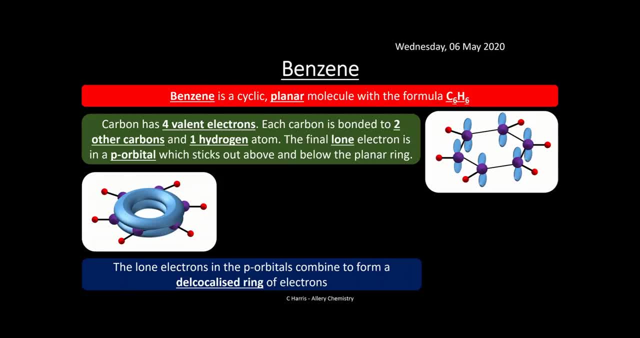 So that sits above and below the planar ring, So you can see it's planar. apart from the orbitals which stick out. Now what these lone electrons do is they actually combine to form a delocalized ring And you can see here it looks like a donut. 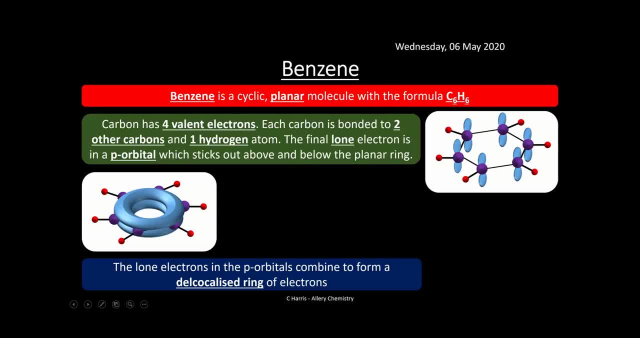 You've got a delocalized ring system here on the left-hand side, And so that's that delocalization actually gives benzene its unique characters, which we'll look at in a minute. So all the bonds, all the CC bonds, in benzene are actually the same length and 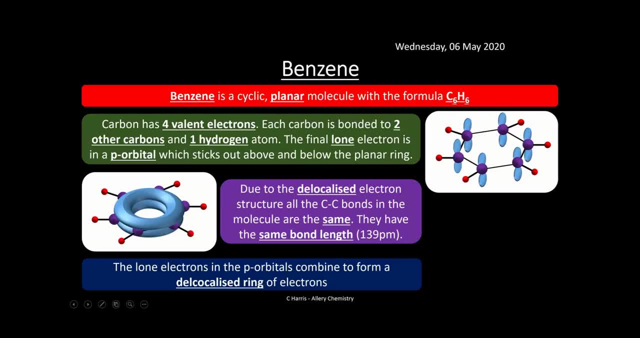 they all have the same length, bond length of 139 picometers. So you can see here that obviously a single bond would be longer than a double bond, because you might have double bonds here, normally single double, single double. And we'll look at that model in a. 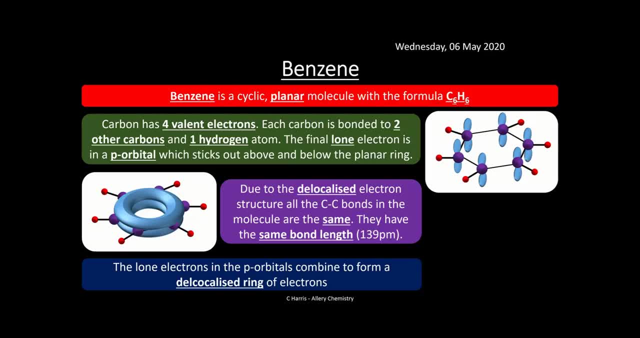 minute and prove why that's not the case. But normally bond lengths are different, but in benzene it's very strange that it actually has the same bond length. So this is what I was saying. So with the single and double bonds, the CC bond length. 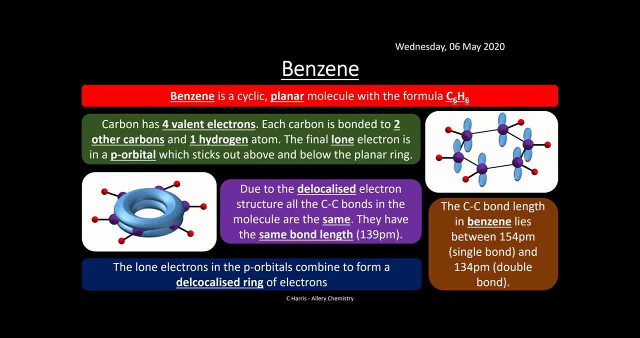 in benzene is normally between 154 picometers for a single bond and 134 picometers of a double bond. So actually it's not a single bond and it's not a double bond. So it has like a unique feature, this benzene. 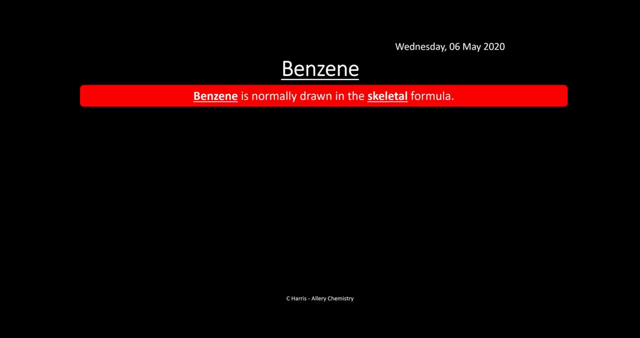 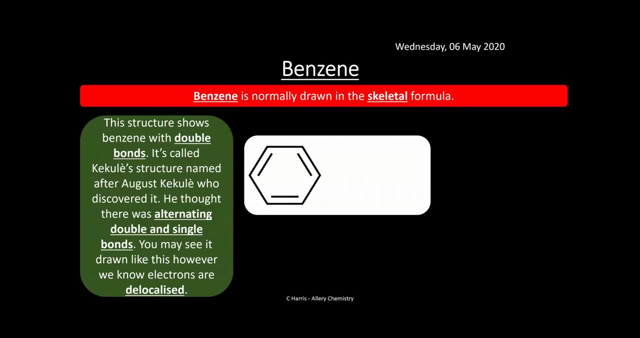 Okay. So basically, Yeah, benzene's normally drawn in the skeletal formula, just because it's a lot easier to draw. there's a lot of atoms in a benzene molecule so it's easier to draw it as a as a skeletal uh formula. so the 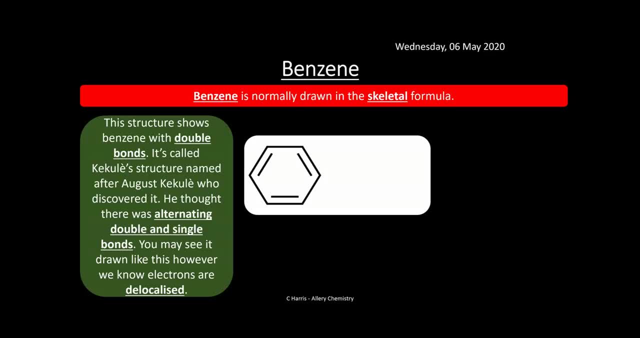 structure. this structure here shows benzene with double bonds and it's also known as a kecule um, a kecule structure. who is? it was named after august kecule, who discovered it, and basically he thought there was alternating double and single bonds, um, and you may see it like this where you 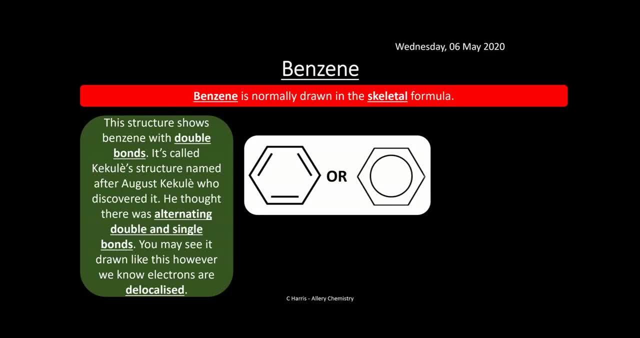 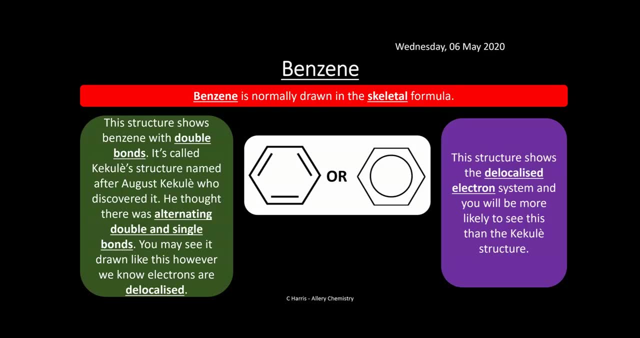 have um alternating single and double bonds, or you can see it like this, where you've got the delocalized system being drawn, so we just draw a circle in the middle um, now in at a level, you'll more likely see it drawn as the one on the right here, which is the um, which is the one with the 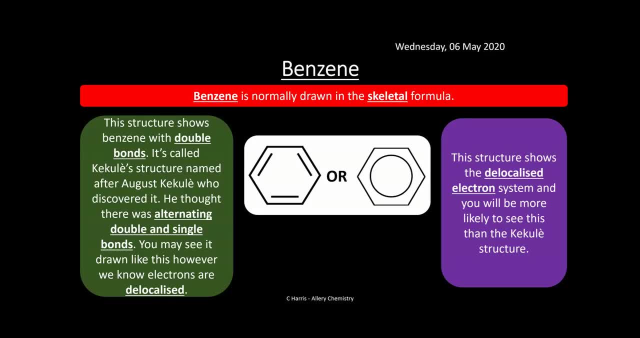 delocalized system rather than kecule structure, although, um, sometimes it's easier to draw um reaction mechanisms using, uh, using kecule structure, but at a level you're mainly going to see is the circle. so that's what i would suggest you draw as rather than kecule structure. so remember, even though 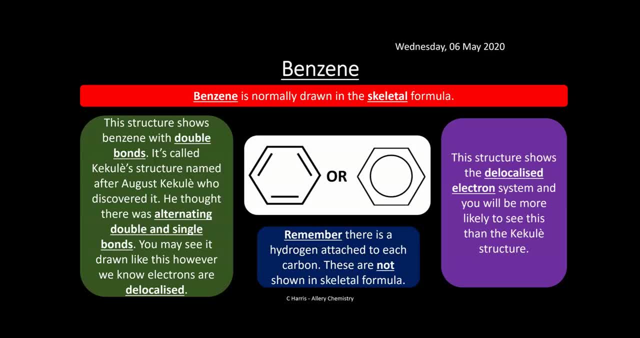 we're drawing the skeletal structure. it's sometimes difficult to spot what atoms are actually in there. but remember, because it's a skeletal structure, hydrogens are not shown in that diagram, um, but there are hydrogens attached to each carbon. so each point on this, on this hexagon here, has a 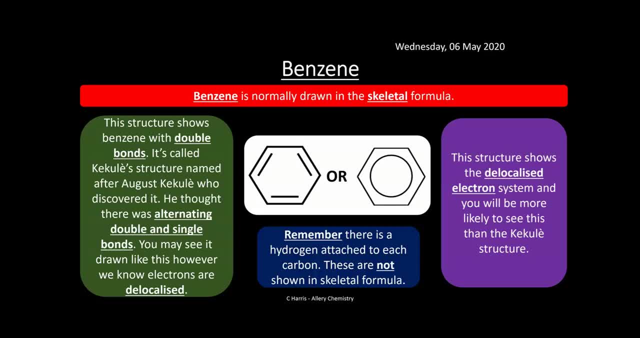 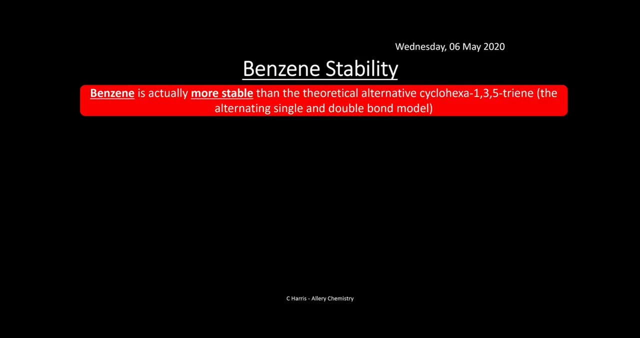 hydrogen hanging off it as well, but we don't show them, obviously, in skeletal formula. okay, so let's look at the stability of benzene. so actually benzene's more stable than the theoretical cyclohexo 135 triene, that's the one with the 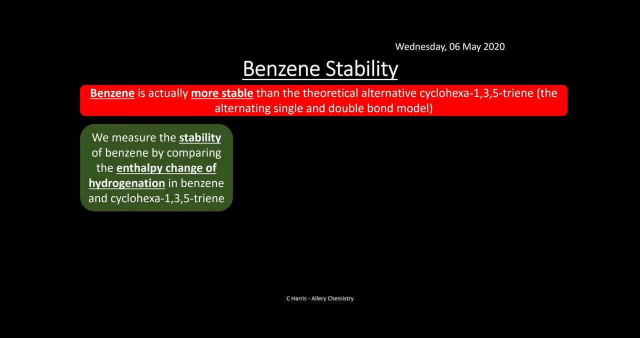 three alternating double bonds, um so, and actually scientists have um, looked at um scientific evidence, um, and that could be through chemical reactions, x-ray crystallography, etc. so what they've done is they've actually looked and thought: well, actually it's more stable than than we, and 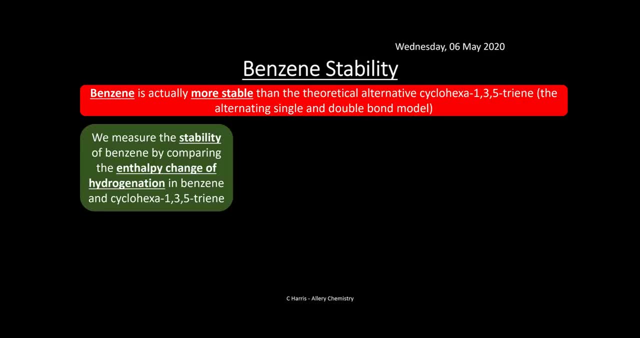 then we think: and it doesn't have this 135 triene structure or the stability of that. so we measure benzene by comparing the enthalpy change of hydrogenation in benzene and cyclohexo 135 triene. so hydrogenation is basically just adding hydrogen to something. so if we add high, if we hydrogenate, 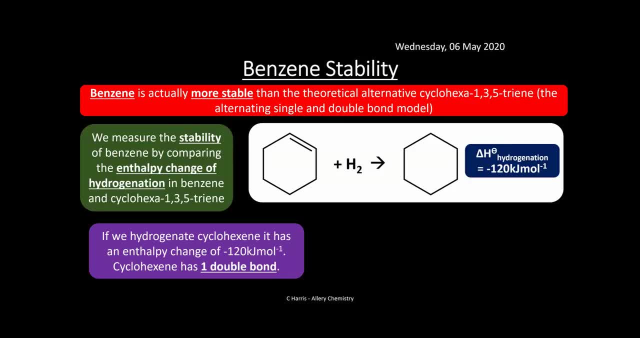 cyclohexene. okay, it has an enthalpy change of minus 120 kilojoules per mole. so basically, cyclohexene has one double bond. so we're looking at right. how much energy does it take to add a hydrogen molecule to, or hydrogen to a double bond in a cyclic compound? and from um from practical experimentation? 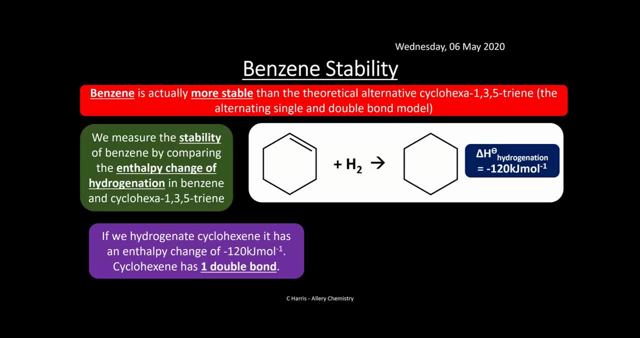 we see that the enthalpy change is minus 120 kilojoules per mole. so if benzene did have the three double bonds, like calculate thought we had, then surely we would expect the enthalpy of hydrogenation to be three times that. so it'd be three times 120, which is minus 360. that's what. 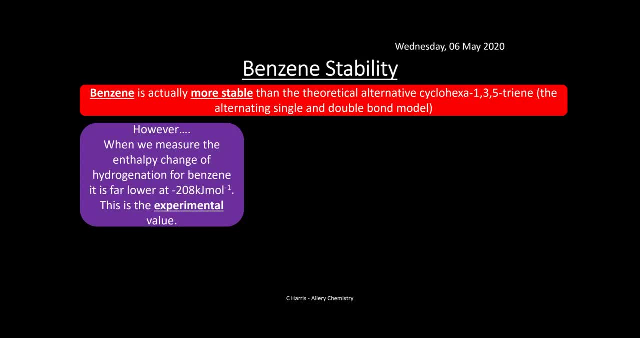 we would expect if it had three double bonds. however, when we measure the enthalpy change, hydrogenation of benzene, we actually get a value that's much lower, which is minus 208 kilojoules per mole, and this is the experimental value that we've actually calculated when working out with benzene, when we're actually adding hydrogen to. 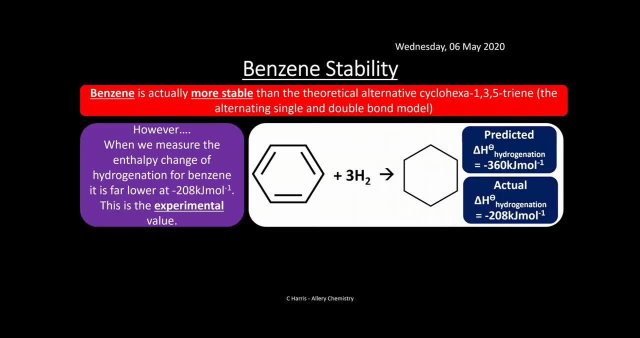 benzene. so we can see here that predicted, if it had the three alternate and double bonds, we would expect it to be minus 360 kilojoules per mole, but actually it's minus 208 kilojoules per mole. so what that means is effectively: benzene is more stable um it's more energy is is required to break. 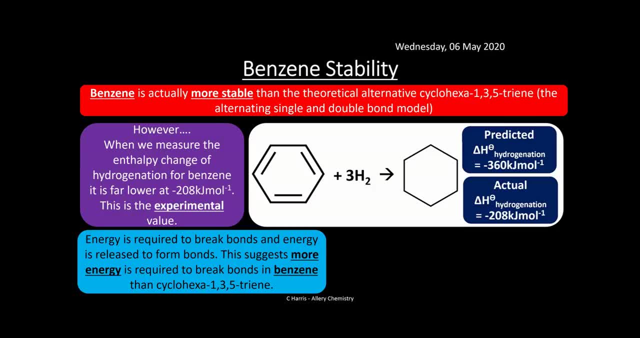 the bonds in benzene than it is in cyclohexane 135 triene. so that means that benzene is a more stable molecule. because we need energy. energy is needed to break them bonds um, and energy is, so more energy is required to break the bonds and energy is released when we actually form them. so 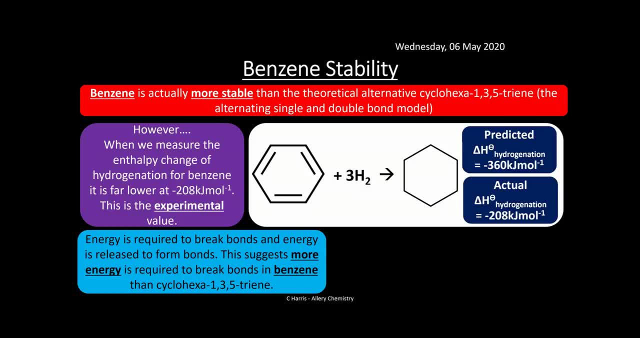 so if it's got a lower energy, it's more stable and it's more stable. so if it's got a lower energy, if it's got a lower enthalpy value, it means it's more stable. so it's more stable, um, and the stability is due to that: delocalized electrons, so that electron system within the benzene ring. 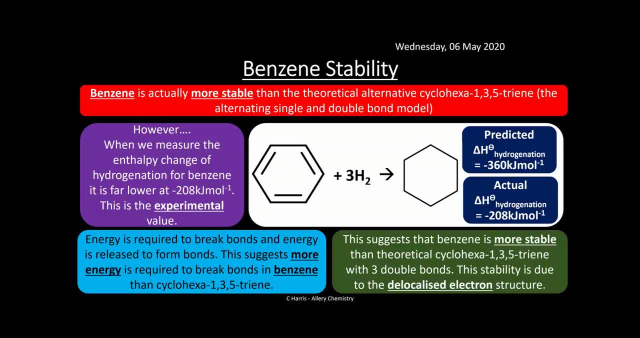 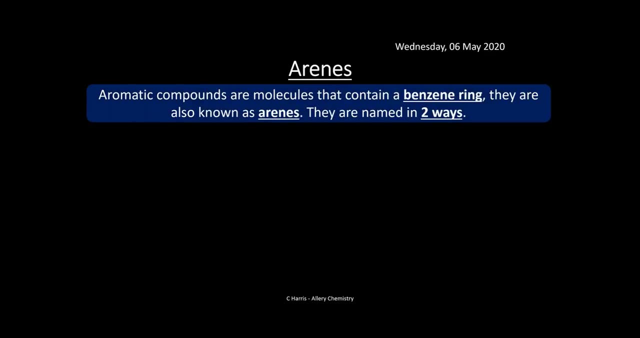 actually increases the stability um and therefore it is. you'll see later. it's actually quite difficult to um to undergo reactions with benzene for this reason. so let's have a look at um arenes now. arenes are a lot more stable than benzene. they're more stable than benzene. they're more stable. 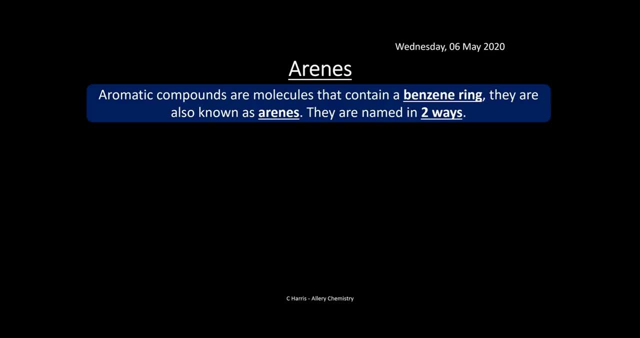 and so these are still there, so we could have basically a change up on a specific group in some of thesecents. but as a side note, benzene is are another word to describe a substance with a benzene ring in it, and benzene obviously on its own is fine. we've seen it there, but actually we 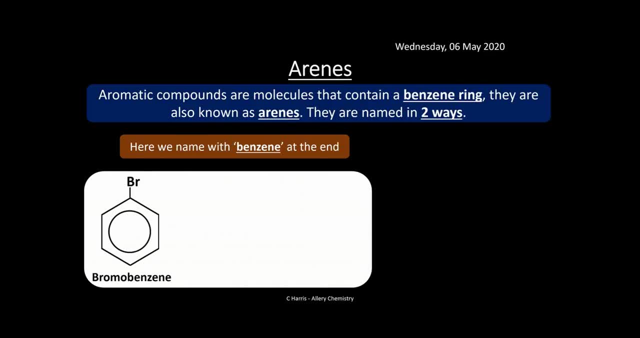 can add groups onto a benzene ring and this is vitally important because it is in loads of pharmaceuticals. um use a rems in there so we can name them in a particular way. so here we go. here's one. here is an example, and we'll come onto these. we'll see the reactions of these later on, but it's. 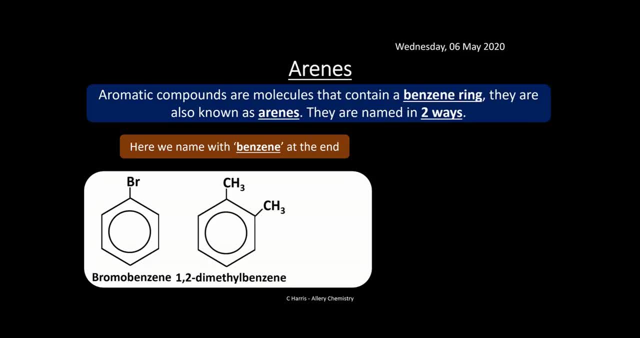 at the end. so, for example, bromo benzene and want to dimethyl benzene. now the numbering of benzene rings. you just pick any number, because it's a circle. we don't really need to know exactly where carbon one is or two, we just assume it's. 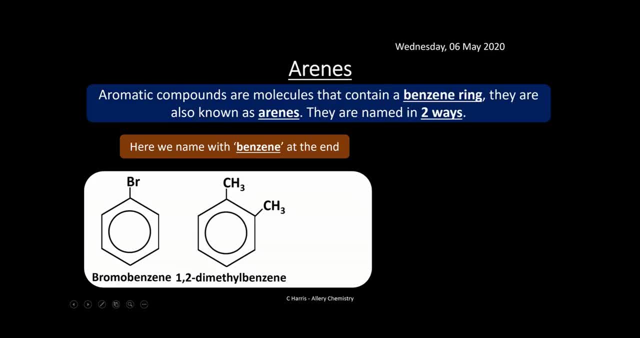 one, two. so you always pick the lowest number and, just like you would do with any other molecule, we number it in the lowest way. so that's one, two and then, once you've labeled, obviously one and you found where one is, then the other one. if there was one here, that'll be four and that'll be five, that'll be six. 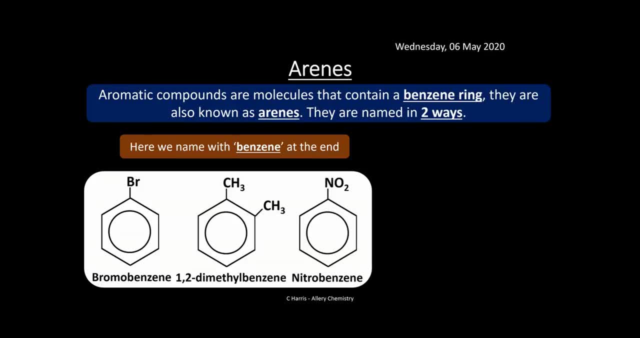 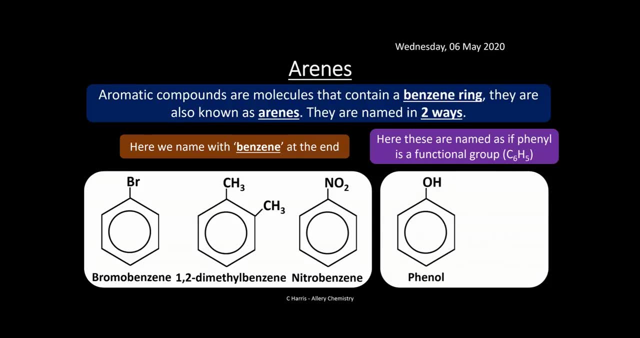 etc. and then nitrobenzene is a is another one. now sometimes you can have ones named as phenyl groups. so here we've got phenol- and we'll look at phenol later on in a little bit more detail- and phenol is basically just a. 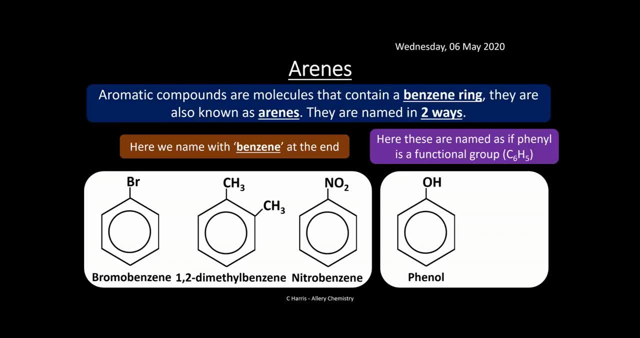 benzene ring with a OH group on the end, but we call it phenol for some reason, so we call it phenol. but for example, you might see molecules such as phenol amine, which has an amine group attached to a benzene, a benzene ring, but we call 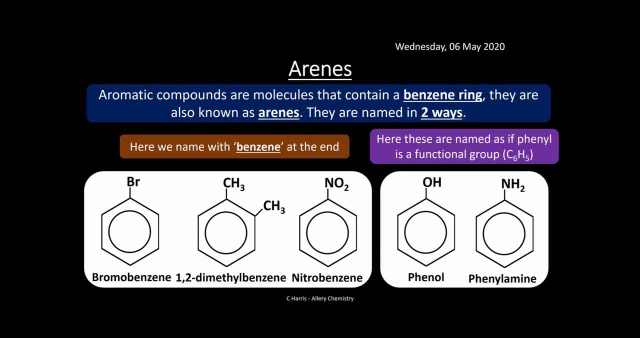 that phenol amine, so just be familiar with the naming of them. sometimes it would be nitrobenzene, bromobenzene, for example, and sometimes it'll be amine at the end, but luckily there's a limited number of molecules that you need to. 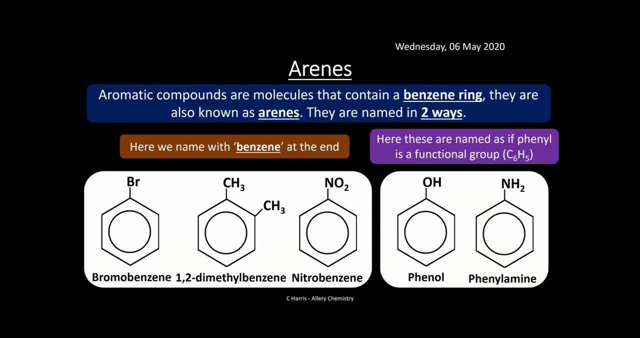 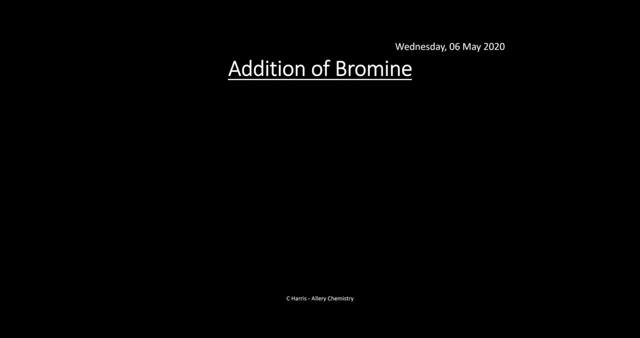 know, and a good start would be the ones that you see right in front of you there that you need to remember. okay, so let's look at, because we've looked at benzene and benzene has double bonds. what we need to try and do is look at the, the, 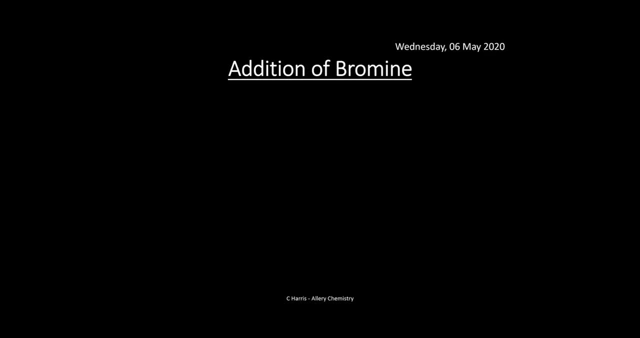 different types of reactions, how benzene reacts. but what we're going to do first is look at normally, how do reactions happen on with double bonds, okay, and one of the classic examples is: added bromine to an alkyne, so alkenes have a double 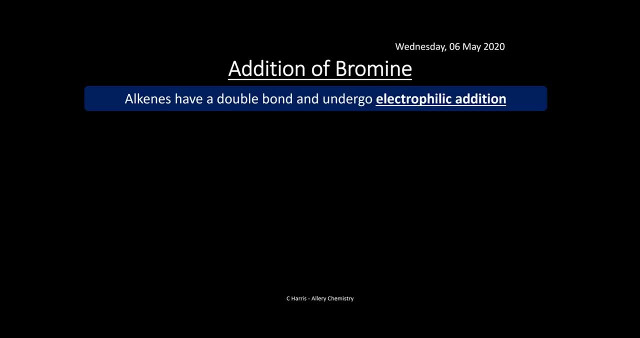 bond and they undergo something called electrophilic addition. okay, so if we have bromine water to an alkene, is a color change from brown, a brownie orange, to a colorless solution. now you might have done this practical actually, where you've done a test for an alkene or test for a double bond, and that's where 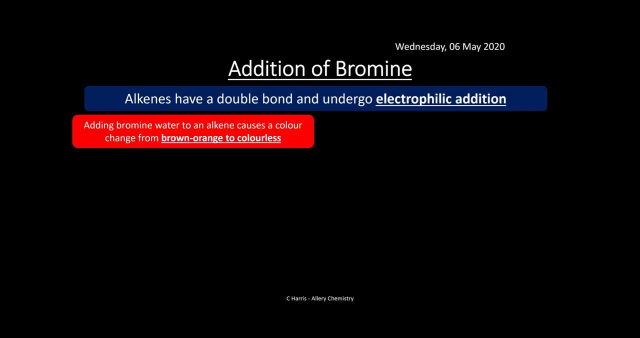 you add bromine water to it and it decolorizes bromine waters. you might have done that already, you might have seen that, but basically the bromine is the electrophile. okay, so remember what an electrophile is, and you might have done this from from. you certainly will have done it in year one. 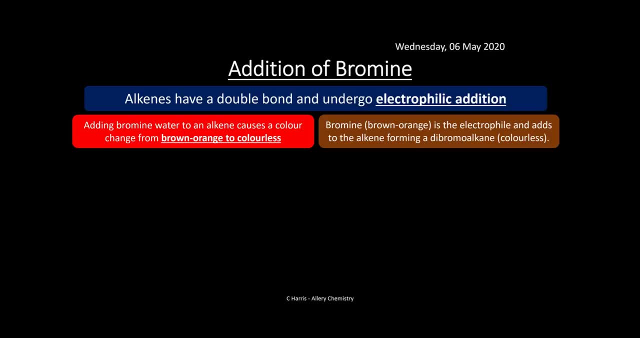 um. so if you're not sure, go and have a look back. i've got videos on um in the year one playlist, um ocr year one playlist. have a look back there to see what an electrophile is. but an electrophile is an electron loving species. so it's a species um which will um attack something with a high. 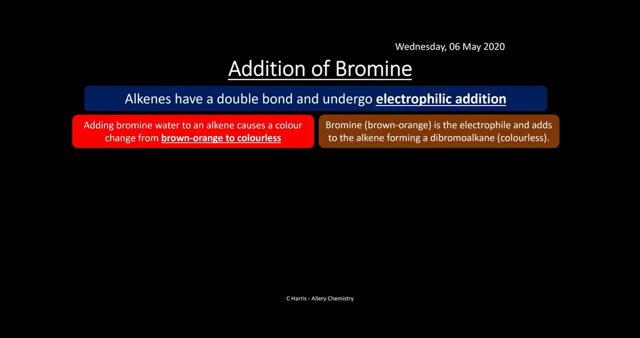 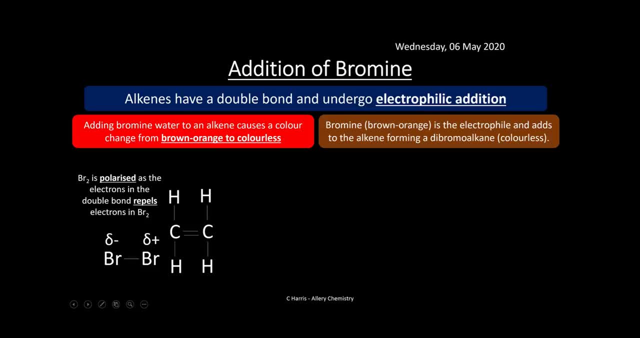 bond and we have a polarized um molecule, so it's an induced, induced polar molecule. as it approaches this double bond, we get electrons in this bond moving to one side of the molecule because of electron repulsion. so there's loads of electrons in that double bond there, and so what happens is: 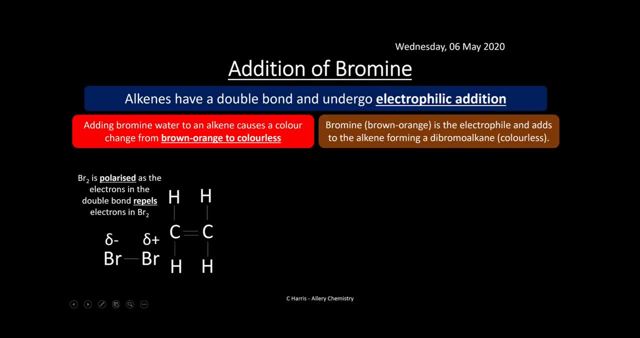 the electrons move to the left hand side and they bunch up onto the bromine and so we get repulsion. now the electron pair in the double bond is actually attracted to the delta positive bromine molecule, so the bromine atom- sorry on them, on the on the molecule there. and what happens? this breaks that bromine- bromine bond. 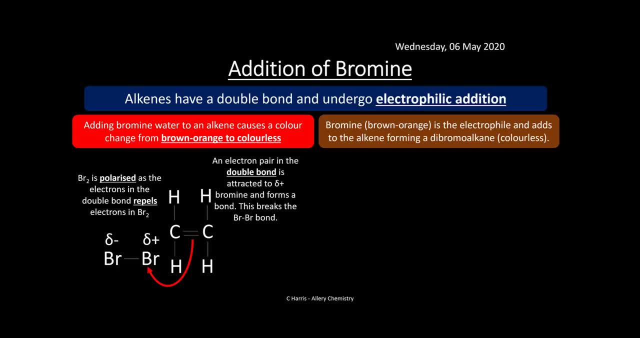 so here it is. so the electrons. remember the curly arrows always show the direction of electron transfer. so the electrons are in that double bond and they're moving towards that bromine, that delta positive bromine. make sure you're drawing arrows correctly again. look back at year one notes. 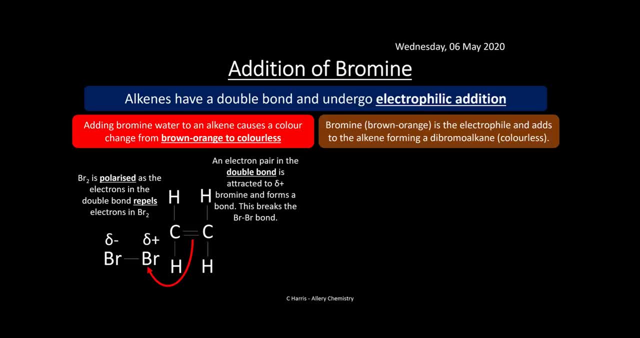 look back the year one videos on an introduction to mechanisms and, because that's very importantly a mechanism, you need to know how a mechanism, how a mechanism works. but it's moving from that double bond into the bromine there and then what effect that is going to have, is going to break that. 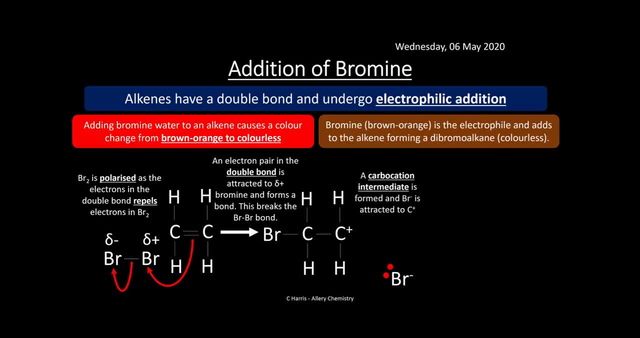 bromine, bromine bond. so we're going to form an intermediate and this is a carbocation intermediate. so you can see, our bromine has been added onto here, so the double bond is now broken, the bromine's added on, but we have a carbon with a positive charge of carbocation. um, we have a br minus because 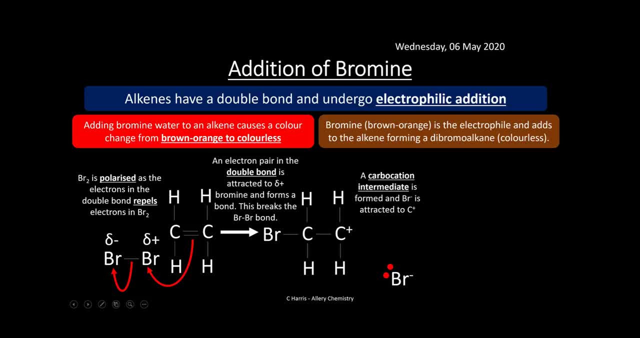 it's this bit here. this is broken off. we have a BR minus. because it was this bit here, this was broken off. we have a. even bronze is broken off. we have a br minus. um, uh, ion, that's moving around freely. now that is effectively going. 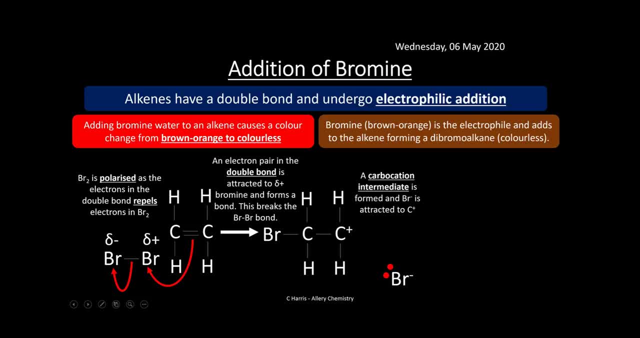 to react with this. so what we're going to have is an arrow going from the lone pair to the positive charge on that carbon, and it's going to try and form bond with that carbon. so here we go, there it is. so we're going to form a colorless compound, which is one. two dibromo ethane is formed, so 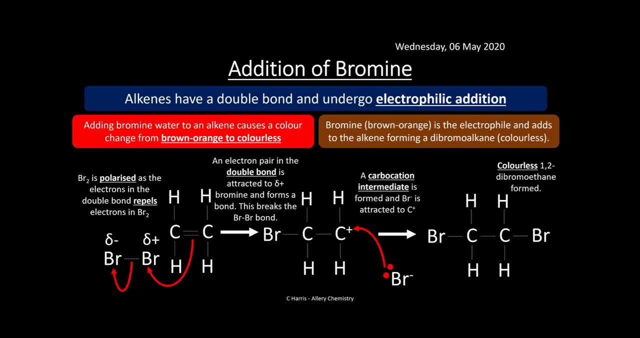 effectively, we've broken that double bond and we've added bromine to it. so that's the basic mechanism. so it's electrophilic addition, because the bromine is the electrophile and we're adding it to a double bond. okay, so these are the standard reaction mechanisms for anything with an alkene. so 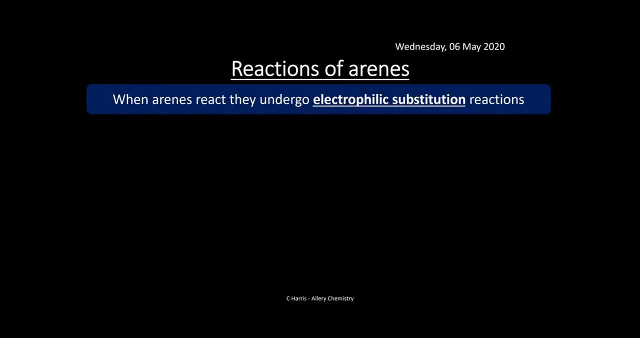 anything with a double bond. now arenes undergo a very different type of reaction and although we've seen there they could have double bonds, the double bonds, the electrons that would form double bonds, actually delocalize into a ring and that completely changes the type of reactions. 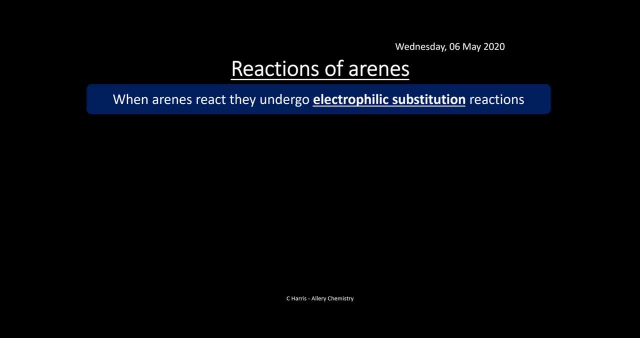 that you can do with benzene, and actually they undergo electrophilic substitution. so this is why it's important to show you what reaction is with an alkene and contrast that with what a benzene reaction would, um what benzene reactions typically are. so benzene has a really high electron density. 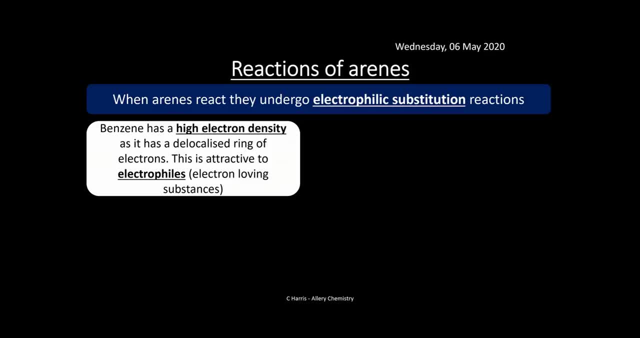 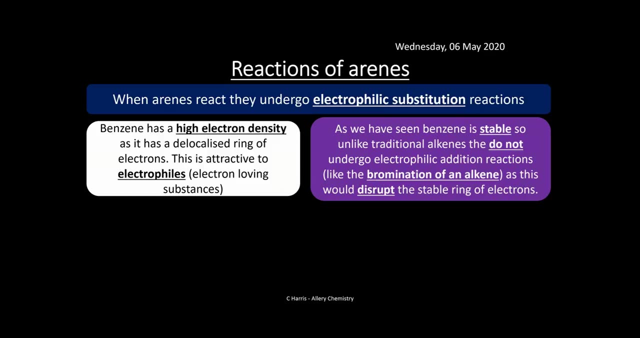 in that delocalized ring. there is loads of electrons in there, so this is attractive to electrophiles, so these are electron loving substances. okay, so that's the key thing. so, as we've seen, benzene is really stable, so remember that from from from what i mentioned before. so, unlike traditional alkenes, if you've- 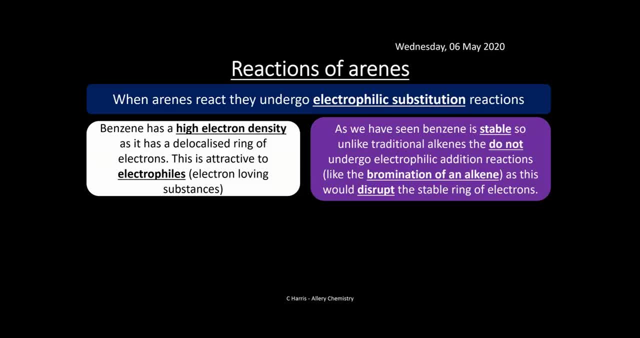 seen before. they do not undergo electrophilic addition reactions. um, and because what will happen is this will disrupt the stable ring of electrons, and one of the things that we know from chemistry is atoms are incredibly lazy. they don't want to be put in a position where they're less. 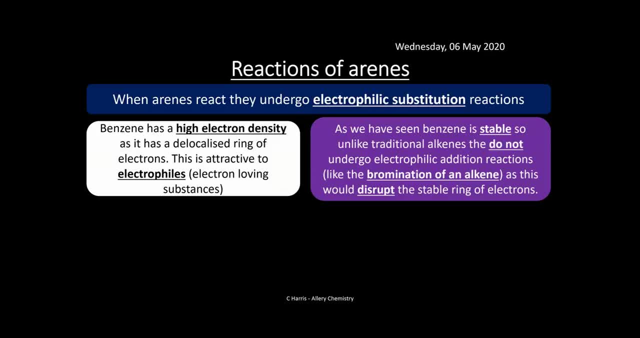 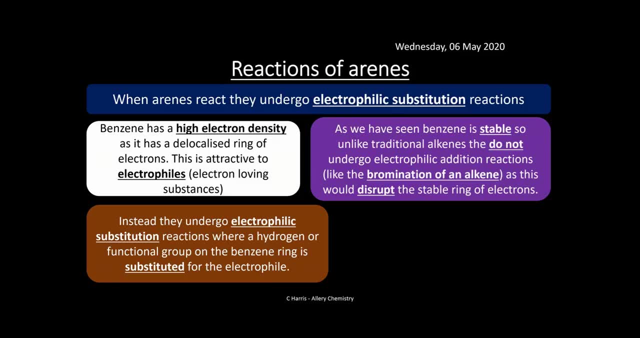 stable, if you know, if possible, unless they're forced to um so. so they don't undergo addition for that for that reason. so what they do is they undergo substitution reactions instead, and this is where um, a hydrogen, one of the hydrogens on the benzene, is replaced for another functional group, um, and this functional group. 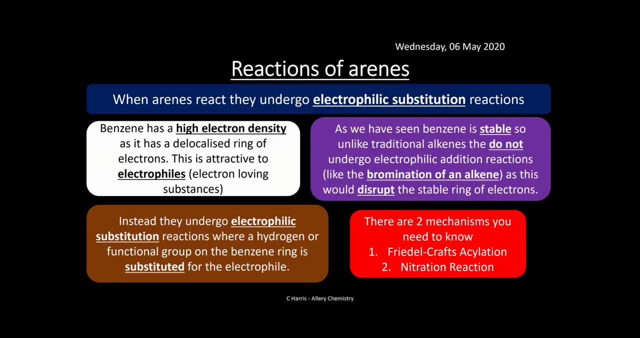 would be the electrophile that we're reacting it with. and there's two mechanisms that we need to know for ocr: one is a friedel kraft's acylation and the other one is a nitration reaction. so we need to know how they react and and how, um and how they react. so let's have a look at the first one. 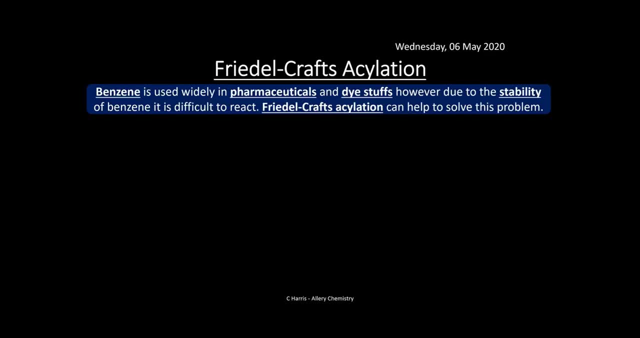 which is friedel kraft's acylation. so benzene is is a massively- as i said right at the start, benzene is a massively useful uh chemical that is used in pharmaceuticals. it's used in um dye stuffs um. it's used in um pesticides, for example herbicides, so it can be used in various different 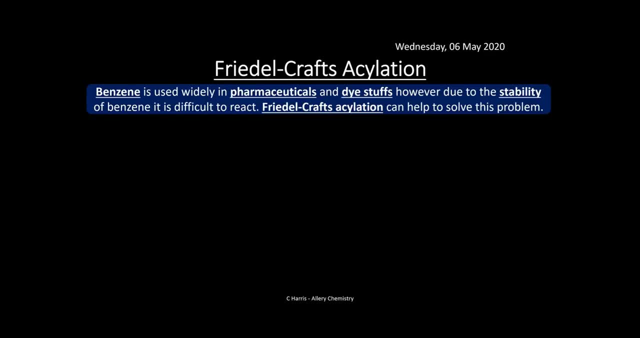 forms and it is. you know, without it we wouldn't. we wouldn't have the things that we do have today. but due to its stability, benzene is really difficult to react. um, it's not the best molecule if you want a reaction. ideally you want really reactive substances, but friedel kraft's acylation. 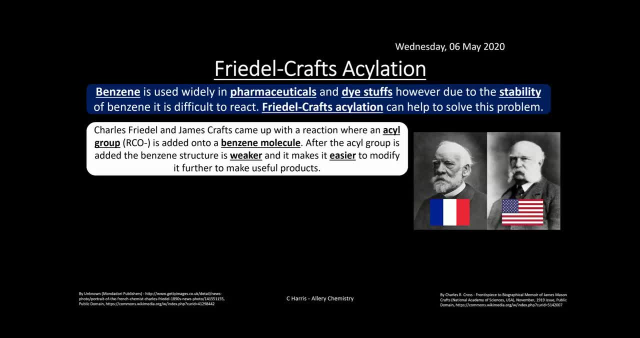 can help solve this problem. so it was left out, these two chaps here, which is charles charles friedel and james kraft. so um friedel was um was french and james kraft's was was american. and and what they did is they came up with a reaction where an acyl group okay, which is this: 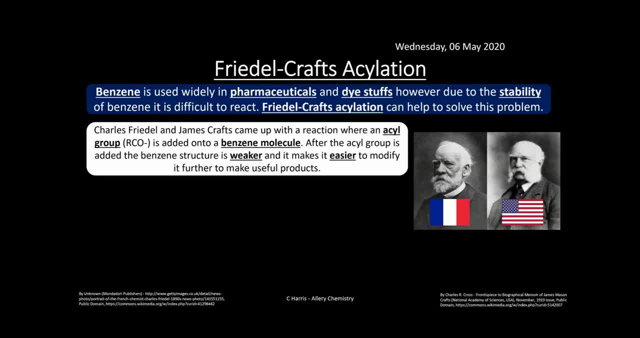 oh, is added onto a benzene molecule, um, and after that's added the benzene structure is weaker and it makes it a lot easier to modify it. so once you've broken into that into that first, once you've substituted your first hydrogen, the rest of the benzene ring is much more susceptible to. attack from other species, so it's actually a really, really important reaction. so, um, in order to get onto the benzene ring, the electrophile must have a very, very strong positive charge. it's no good just having a delta positive, like we've seen with the bromine molecule. 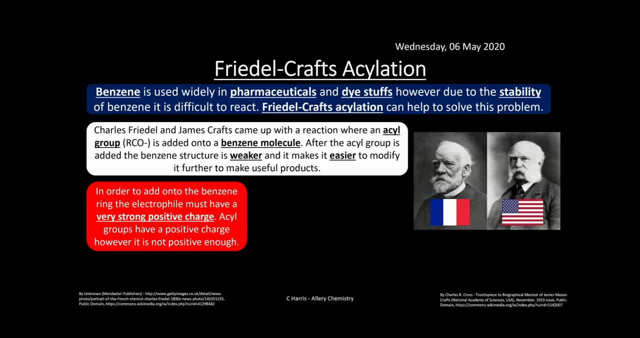 we must have a really strong positive charge here, because if we're going to attack this ring, we need something that is really, really powerful. okay now, acyl groups have a positive charge already because they have that um, delta uh, delta, negative, delta, positive, um uh interaction with. 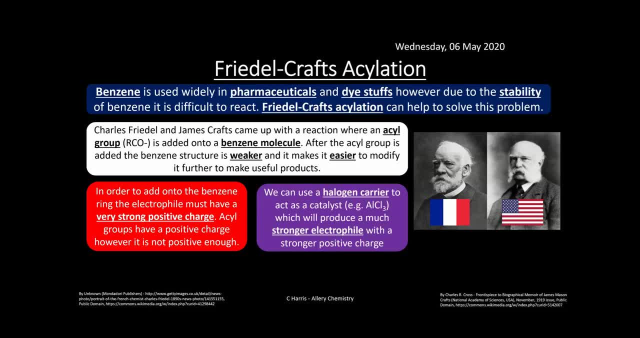 the carbon and the oxygen. however, it's nowhere near positive enough. so what we use is we use a catalyst, and this will allow us to produce a much stronger electrophile with a much bigger positive charge and that is powerful enough to break that um, that barrier of um substituting. 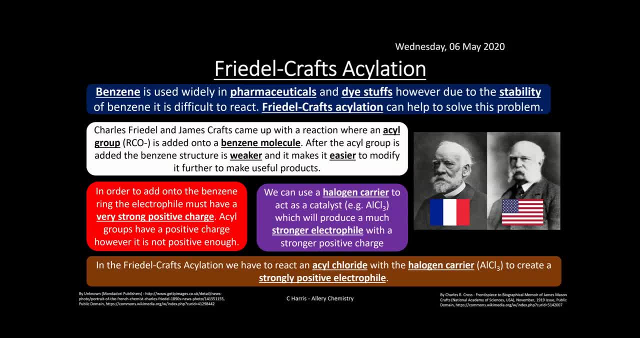 hydrogen with with your functional group. okay, so in the friedel crafts acylation we react an acyl chloride with a halogen carrier which is alcl3, and we create a strongly positive electrophile. so let's have a look and see how this works. 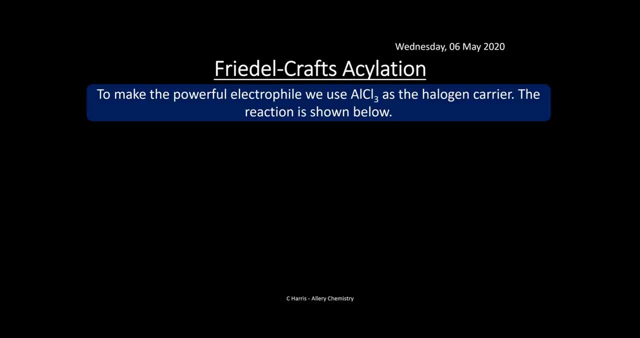 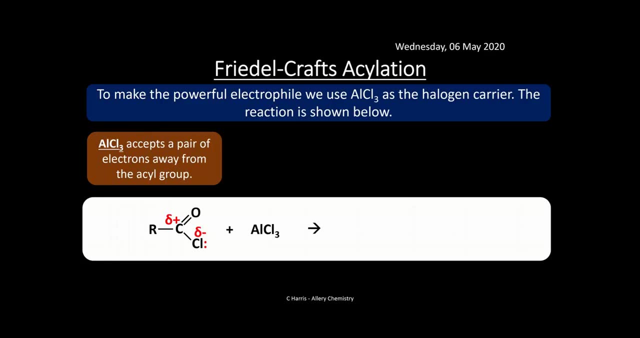 practically so. to make this, we have to use aluminium chloride, so alcl3, um, which is your halogen carrier, and we basically do this first. so our alcl3 accepts an electron away from the acyl group. okay, so here's our acyl group here on the left. so this is here. so this is our acid chloride. 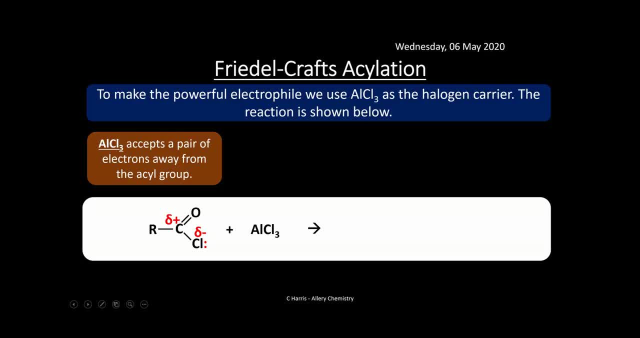 or acyl chloride, and then we have alcl3, which is our halogen carrier. so what happens is we get um the polarization. so, as a result, the polarization increases and the carbocation is informed. so what happens is the chlorine on here now moves on to the alcl4 and we now have a carbon. 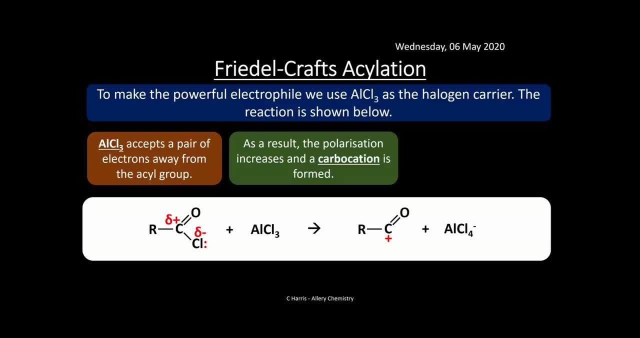 which is heavily deficient in electrons, and it actually has a positive charge. it's not just a delta positive, it is a full, fully blown positive charge. there's a carbocation now that is a lot more powerful um, and that means it will be able to react with benzene quite readily. so that's the 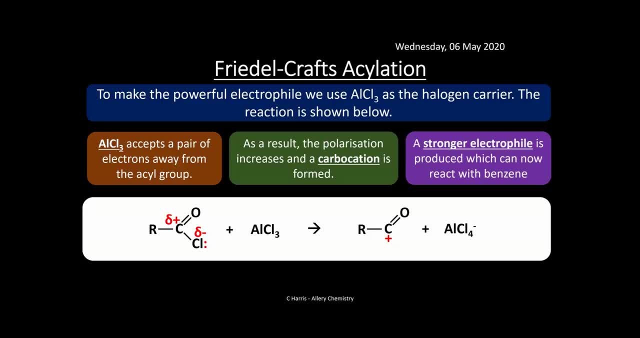 thing with benzene. we have to make a very powerful um electrophile, and this is how we do it, and this is how the halogen carrier- hence the word halogen carrier- what it's doing is: it's carrying the halogen from um, from your um acid chloride, and it's this that's then going to react with your. 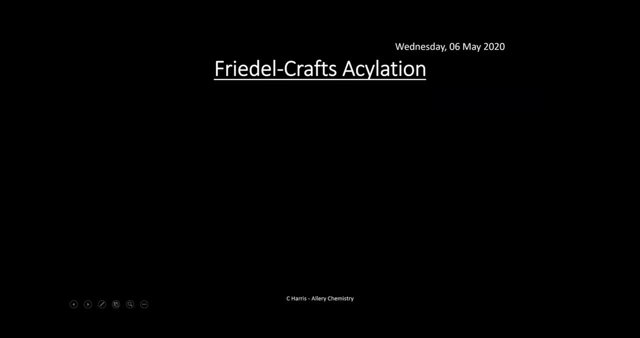 benzene, because that's now got this really good positive charge. so we've made that electrophile. we need to now react it with benzene to make our- um, our stable phenyl phenyl ketone, um, sorry, to make a less stable phenyl ketone, uh, under reflux and a dry ether. 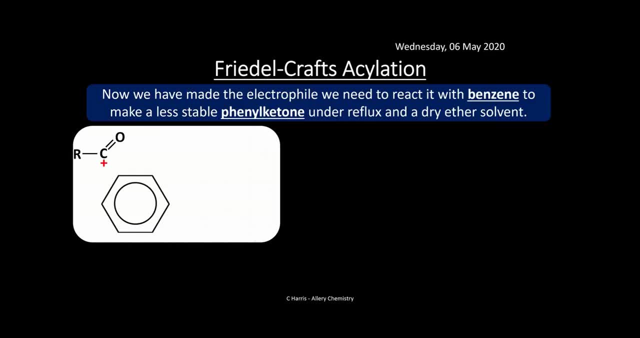 solvent. so the phenyl ketone is what we're making here, okay. so here it is, here, here's our benzene molecule and we've got our carbocation there, which is um, which is our electrophile at the start. so the mechanism goes like this: so we have a delocalized electrons in that benzene ring are 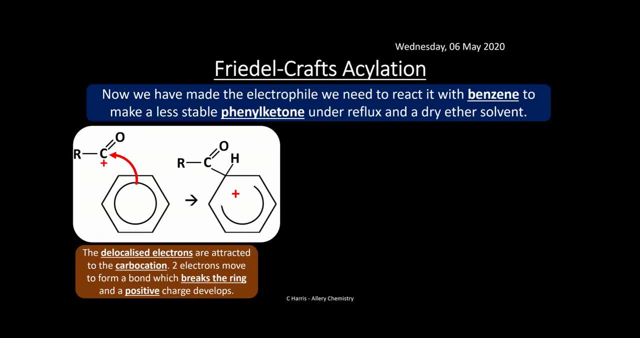 now actually attracted towards this carbocation, because it's it's exactly what benzene is going to react with here, because it's powerful enough so the two electrons move from the bond and that breaks the ring structure and a positive charge develops. so you can see here. 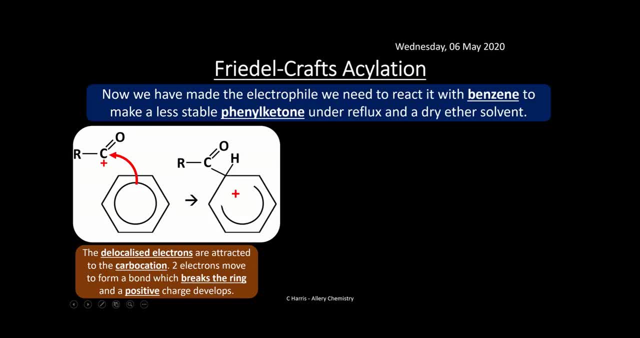 what we've done is we've added our acyl group here, uh, onto the um or the phenyl, sorry, our acyl group here. you've added it onto your benzene ring and the hydrogen is still there. but notice, we have a positive charge. now, when you're drawing these mechanisms, you've got to make sure that you. 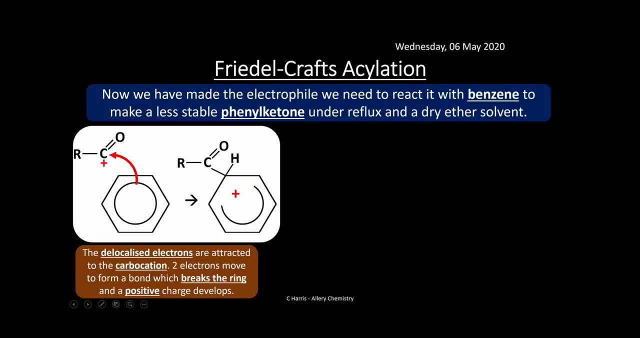 include your positive charge, and you've got to make sure that you include your positive charge. it's very important. and also if you notice that the actual benzene ring has actually been disturbed and it cannot extend beyond this carbon and this carbon, so it can't extend beyond the adjacent. 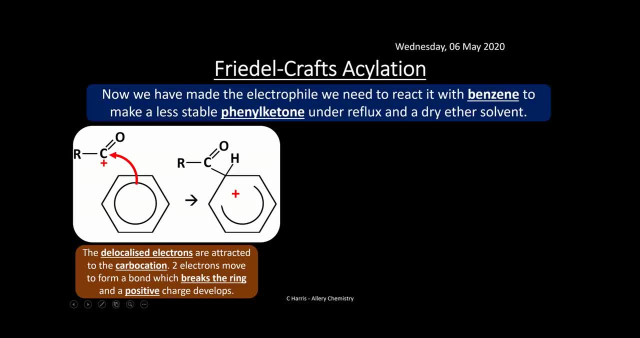 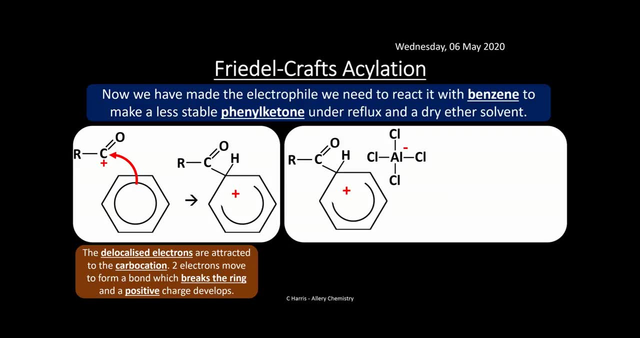 carbons to where the reaction has happened, very important. so you've got to be really meticulous here. so this is our reaction here. so here's our intermediate that we've formed, and remember we also have our halogen carrier that we've, that we've um, that we formed before. okay, remember that. 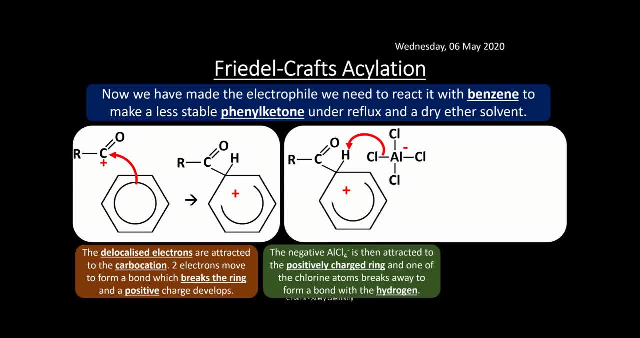 was. that was from the previous reaction. so what happens is the negative alcl4 minus is then attracted to the positively charged ring. okay, because now you've got this, you've got an opposite charge here and one of the chlorine atoms breaks away to form bond with the hydrogen. okay, so you. 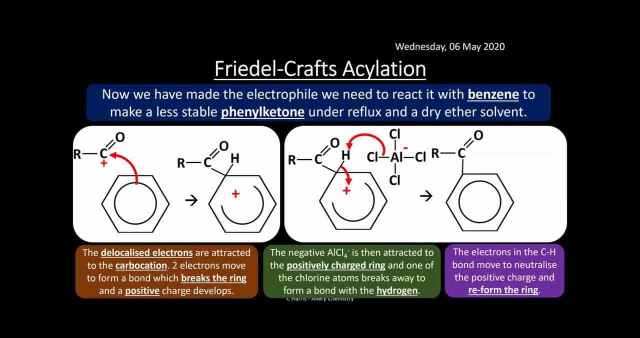 can see here. so we've formed that bond and then what happens is the electrons in the ch bond here then move back into that benzene ring there to neutralize that and we actually reform our ring again, but our hydrogen has now left and our hydrogen is left for the chlorine. so there's 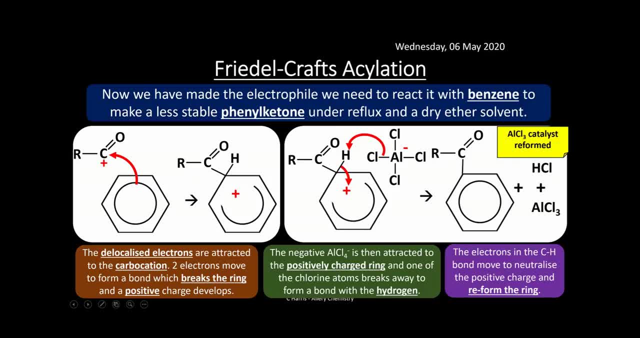 chlorine there, so there's hcl plus alcl3. so we've reformed our halogen carrier back and that is why we call it a catalyst, because the catalyst is never used up. it is reformed in the end. so you can see it's called a halogen carrier because effectively what it's doing is it's just carrying. 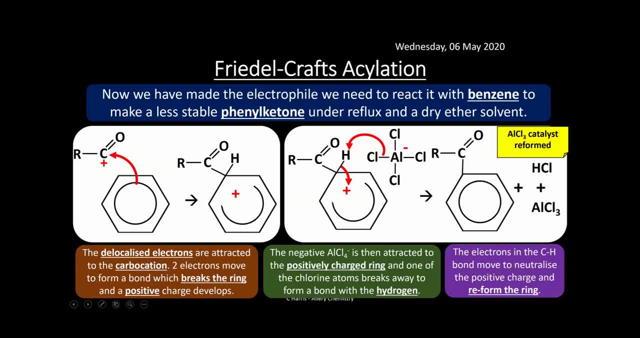 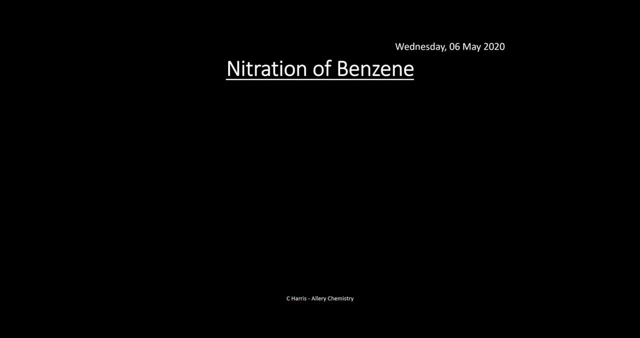 the halogen. until this process here, until this step, when actually the halogen is used to make hcl, okay. so let's look at our other type of reaction, which is the nitration of, of benzene. so nitrate and benzene is useful. it allows us to make dyes and explosives. so, for example, um tnt is tri-nitro. 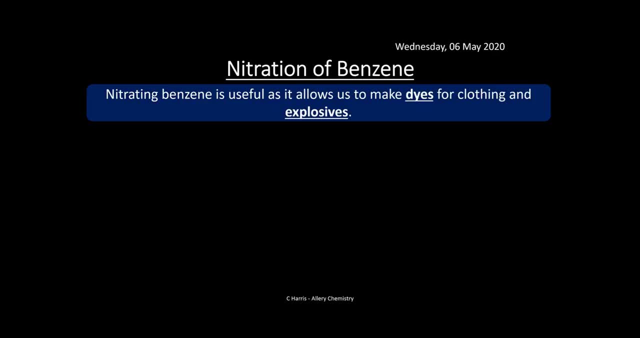 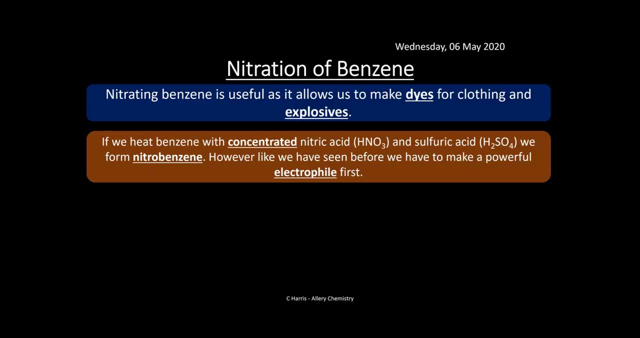 toluene, um and and dyes. you can make azo dyes with that as well, so don't worry too much about the azo dye bit. but we, we do use this. there is a use for this, um. so what we do is if we heat. 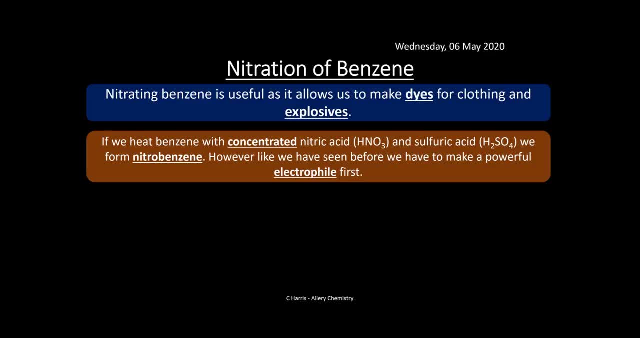 benzene. with concentrated nitric acid and sulfuric acid, we form a nitrogen dioxide reaction to form nitrobenzene. however, just like before, we have to make a powerful electrophile first. it's no good. we can't just take um a nitric acid and add it to a benzene. we have to make a powerful. 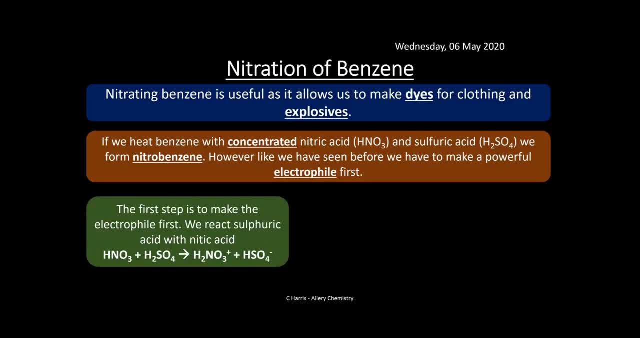 electrophile first. so here's the, the first step. so we make the electrophile, we react sulfuric acid with nitric acid. okay, both of these are concentrated, so they're quite powerful acids, and so what happens is we form h2n03 plus. so effectively, this receives a proton. 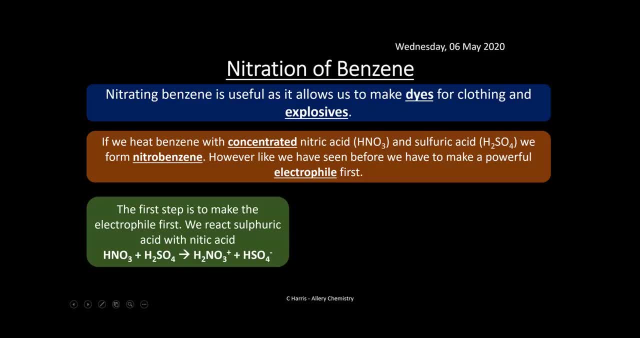 and this donates um, so this loses a proton, so it donates the proton to form hso4. now you would have seen um in the um in the previous videos looking at acids, bases and buffers. if you have a look at that video and then you'll notice that actually, even though both of these are acids- 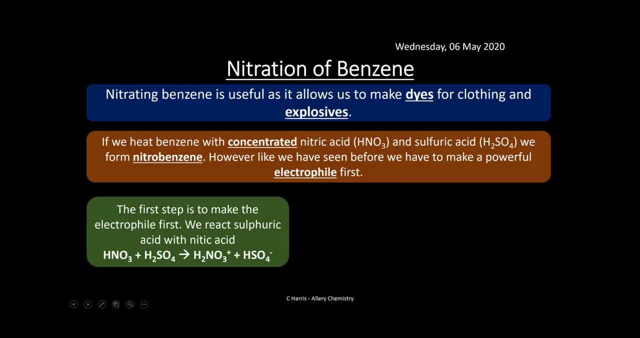 this is a proton acceptor, so the nitric acid is a base. the sulfuric acid is actually acting as an acid because it is donating a proton. so it's funny because nitric acid, even though it's got the word, it's acting as a base in this reaction. so you've got to as long as you know that, um, because that's. 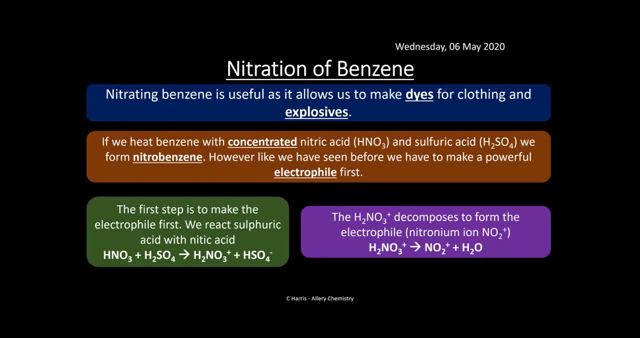 the bronsted- bronsted-lowry theory. so then what happens is that h2n03 plus decomposes to form the electrophile of the nitronium ion, which is no2 plus. so we've got h2n03, which is here that decomposes. 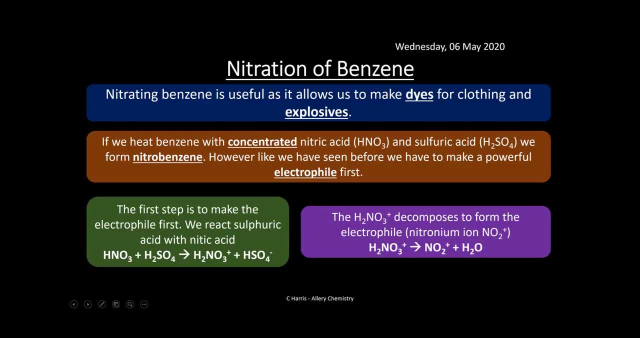 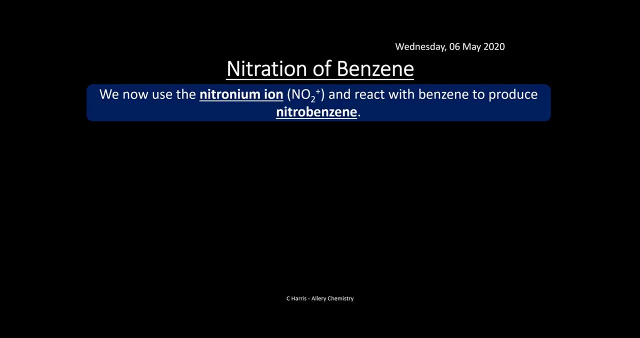 to form no2 plus plus h2o and there you can see, there we have finally, our really powerful electrophile. that's where we want to add on to our benzene ring and it has our positive charge there, okay, so let's look at the mechanism for this. so we're going to use that nitronium ion that we've 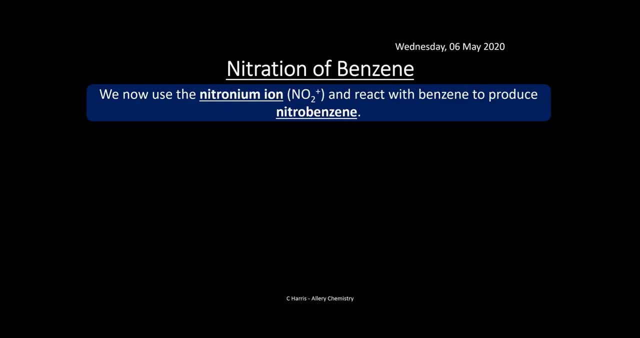 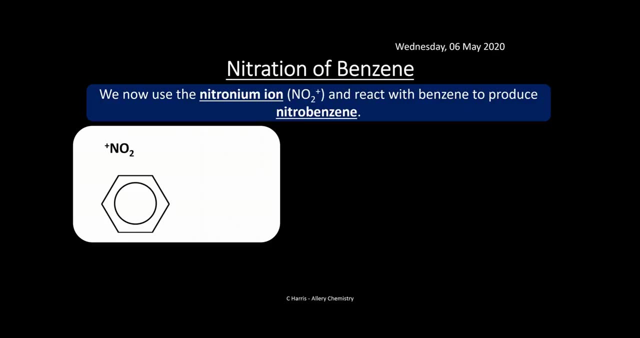 formed there, which is the no2 plus, and we're going to react that with benzene to produce nitrobenzene. the mechanism is the same and you'll see here, apart from the, apart from the halogen carrier, the mechanism is the same. so let's have a look at the first bit. so the nitronium ion is attacked by 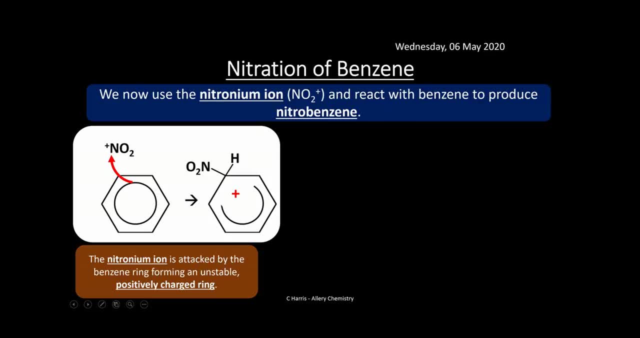 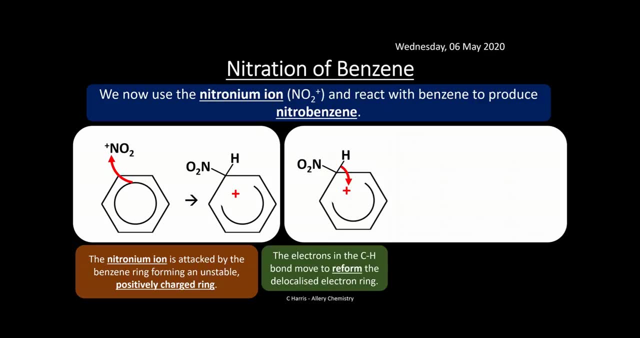 a charged ring, which is this bit. here, and you can see we've added our no2 and there's our positive ring structure. so the next thing is the electrons in the ch bond. here these move to reform the delocalized electron ring. so you can see, there it's, it reforms that back and then what you have. 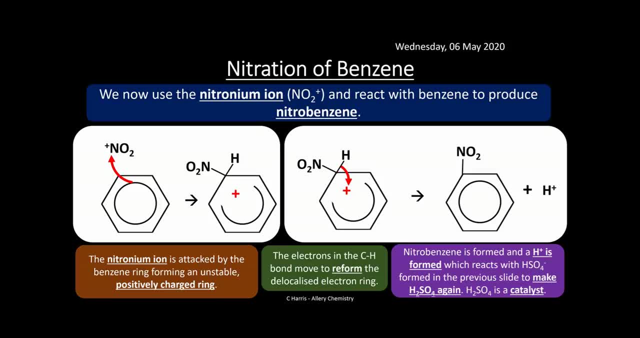 is your nitrobenzene that's formed and h plus ion is formed as well, back now that h plus ion actually reacts with the hso4 formed in the previous slide. so remember the previous one, we had hso4 minus left um and the h that forms h2so4 back again. so actually in this reaction h2so4 is a catalyst. 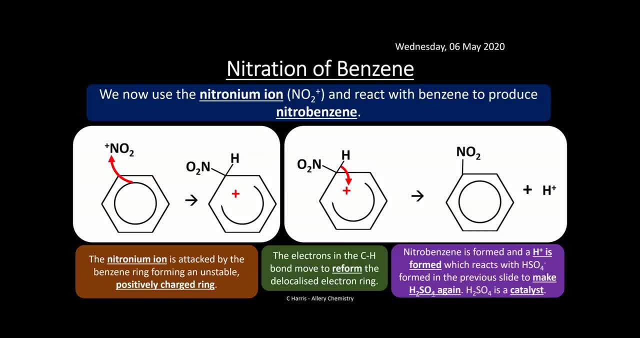 um, so because it's reformed back again. so all these different points here. obviously you need to be able to write the mechanism down and show what's happening, but also you need to identify what's a catalyst and explain why it's a catalyst using your reaction mechanisms. so tie it all in. 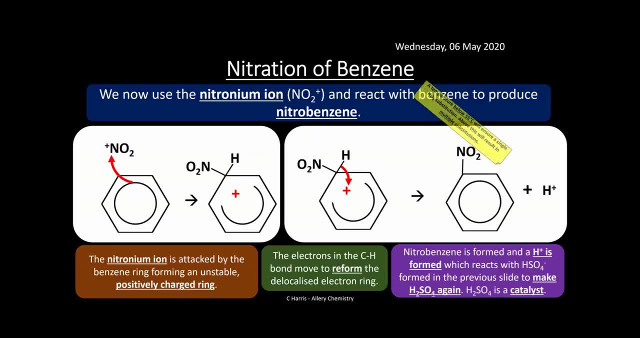 because it all fits together. there's no loose atoms here. so this must be done at a temperature below 55 degrees celsius and this means you get a single nitration um reaction here, right, and nitration substitution um. if it's done above that, you'll get multiple nitration reactions. so you'll get no2 um on carbon 3 on carbon 5 as. 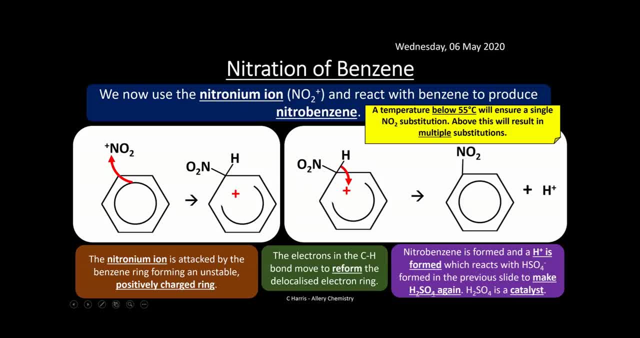 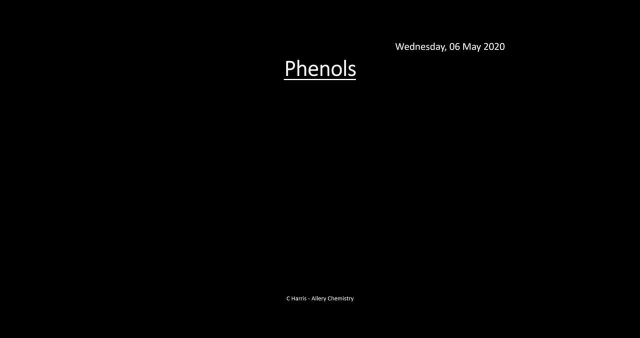 well, so you'll just keep um nitrating it. so you've got to attempt. it's temperature sensitive. you've got to make sure it's done right. okay, so let's look at phenols. when we looked at phenols, well, we introduced it briefly just. 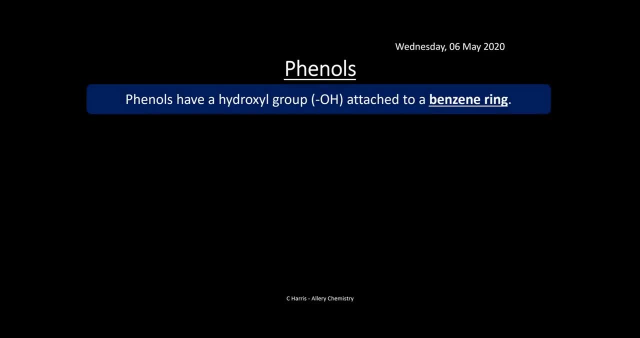 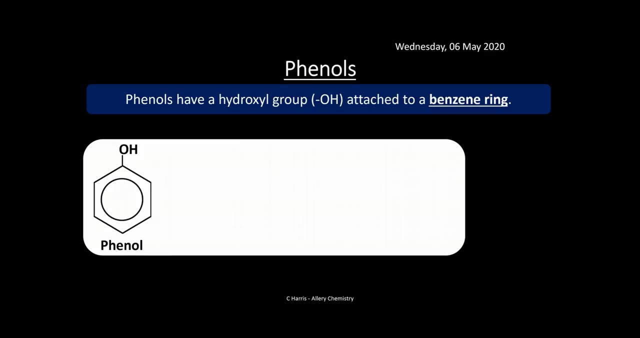 just before um as part of the nomenclature side um. but phenols have a hydroxyl group so it's an oh group and that's attached to a benzene ring. so phenol, remember is um, is a benzene ring with a with the oh group attached at the top there. but we can also get things like two methyl phenol. 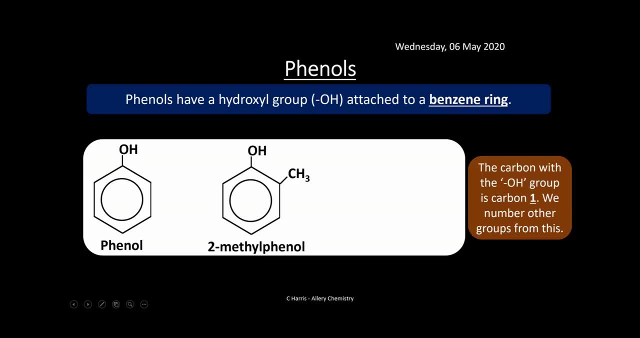 so, for example, we've got a methyl group attached to the phenol um, and the carbon with the oh group is always carbon one in phenols. okay, so that's always carbon one, and so then we go and name it two. now, if it was there, it would still call me two. 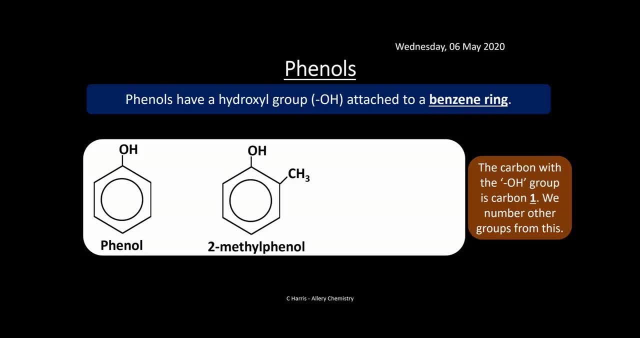 um, because we still be called two, because we always number the lowest number in system. so that's the iupac way. and this one's salicylic acid. um, as you'll, you'll see, salicylic acid, you may see that as well. um later on, um or in, sorry, um, in your um, uh, in your practice, um. 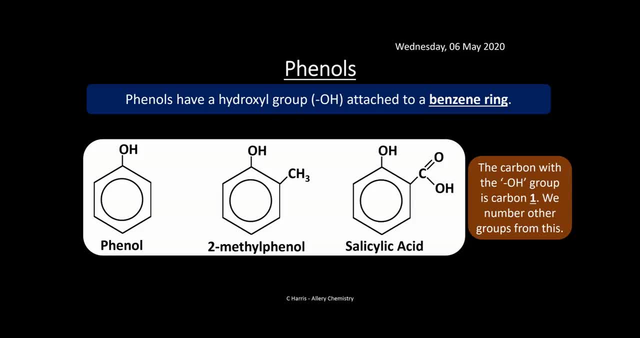 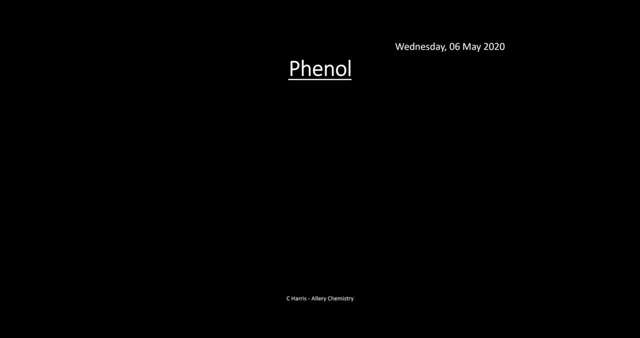 skills. um. salicylic acid is used to make aspirin, uh, which you may have made. so, but that's. it depends if you, um, if your teacher or your lecturer allows you to do that, okay. so phenols are much more reactive than benzene, um, due to their electron density being, uh in the ring being higher, okay. 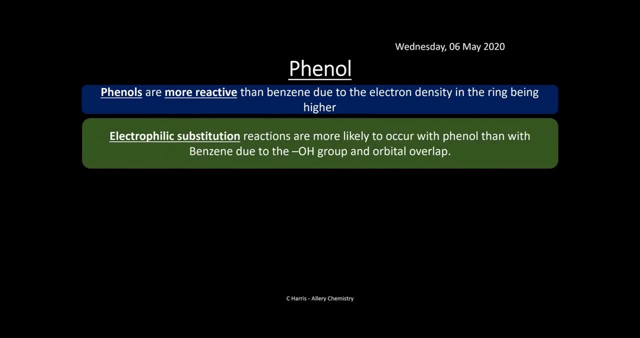 so what we've got is um is. the actual oh group is is donating some of the electrons or pushing some of the electrons it has into that benzene ring. so electrophilic substitutions are much more likely to occur with phenol than with benzene. okay, because of this overall, uh, this orbital 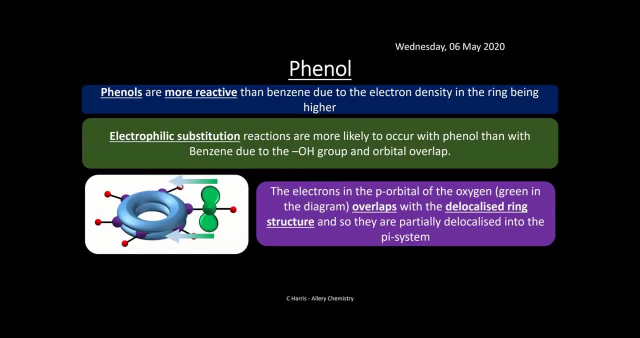 overlap that we've been talking about. so the electrons in the p orbital of the oxygen- so that's the green one here- um overlaps into the delocalized ring structure that we can see there, and so, um, what this does is this: increases the electron density in phenols and, like i say, makes 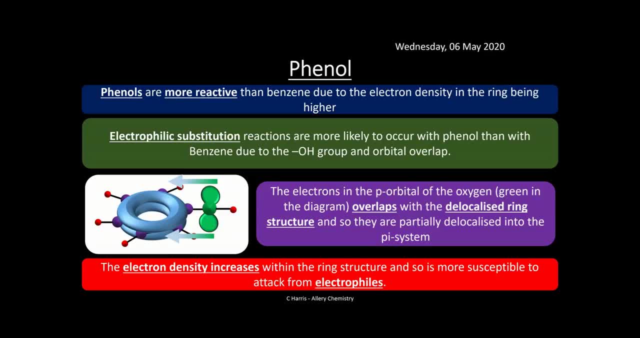 them more reactive, so, um, that means they're much more susceptible to attack from electron electrophiles. um- and this is quite important, because what we're doing is comparing and contrasting reactions of benzene with phenol, and phenol is, is has um far more successful reactions. 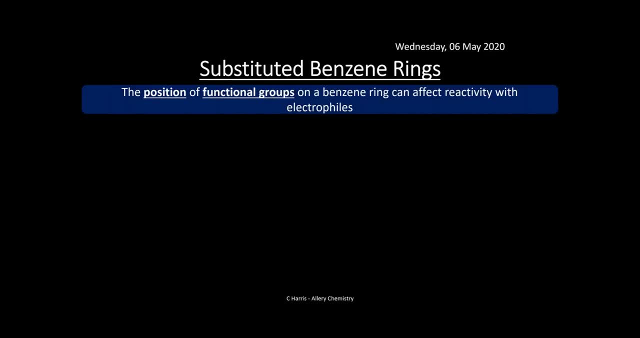 because of this. so the position of the functional groups um in a benzene ring can affect reactivity, um with electrophiles as well. so, for example, benzene has carbons that have the same electron density, so the reactivity is identical to the electron density. so the reactivity is identical to. 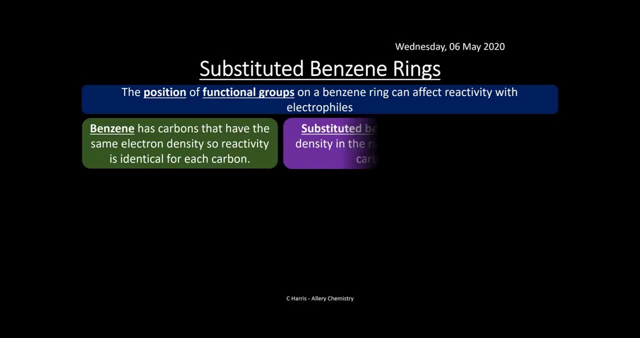 each carbon. so there's no difference there. in benzene, substituted benzene rings distort the electron density, uh and the, and it distorts electron density in the ring and so it affects the reactivity of carbon atoms in the ring as well. so just like with phenol, like we've seen, 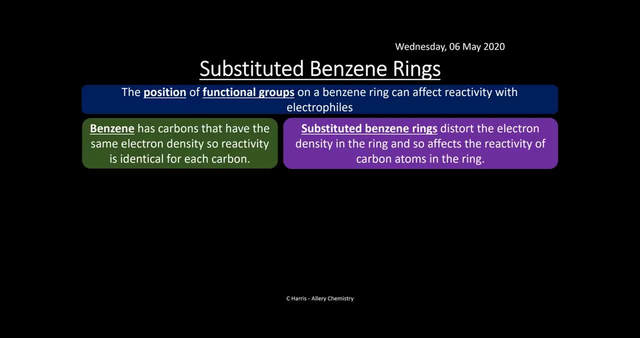 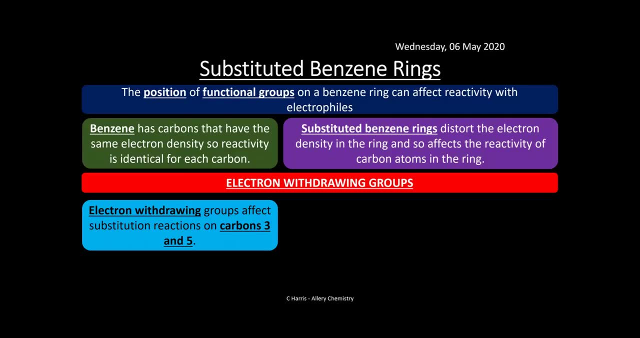 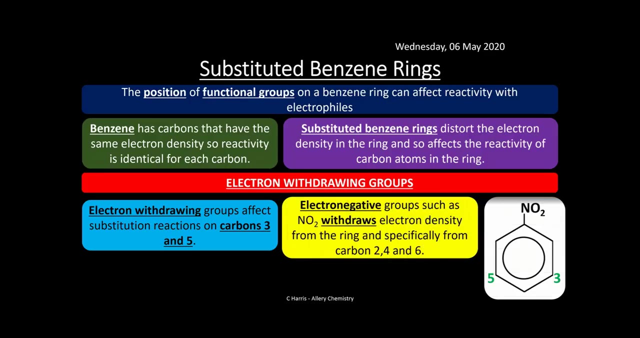 before. that distorts the um, the electron um, the electron movement in the ring. so do other groups as well. so let's look at some electron withdrawn groups. so electron withdrawing groups are effect substitution reactions on carbons three and five. okay. so electronegative groups such as 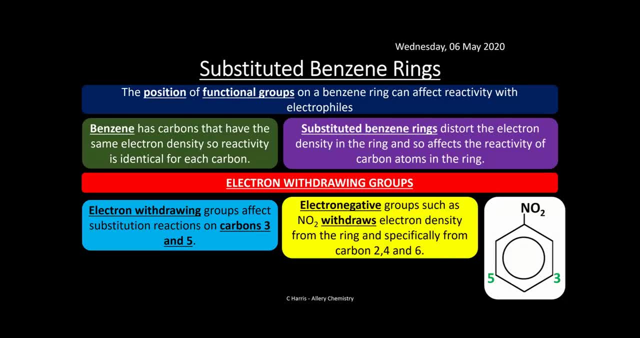 nitrates, for example. as you've just seen before, this withdraws electron density from the ring and specifically, it withdraws it from carbons two, four and six. okay, so you've got to remember that, and so this means your electrophiles are much more likely to attack at carbons three. 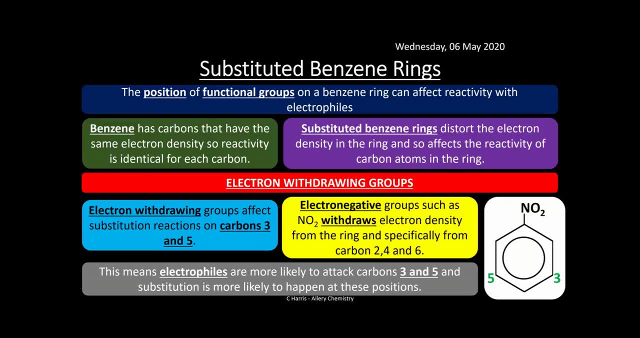 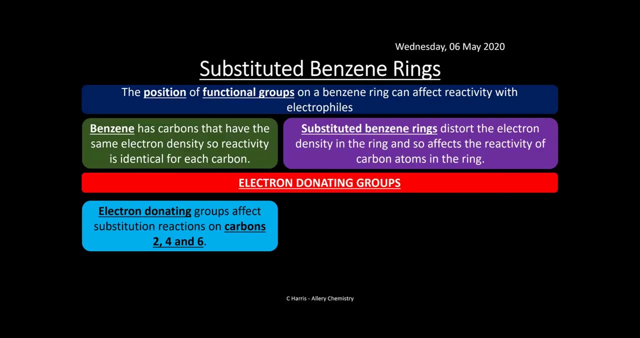 and five um, and so therefore, with nitrates they're more likely to attack at carbons three and five than any other carbon because of the electron withdrawal nature of it. so let's look at electron donating groups. so donating groups affect substitution reactions on carbons two, four. 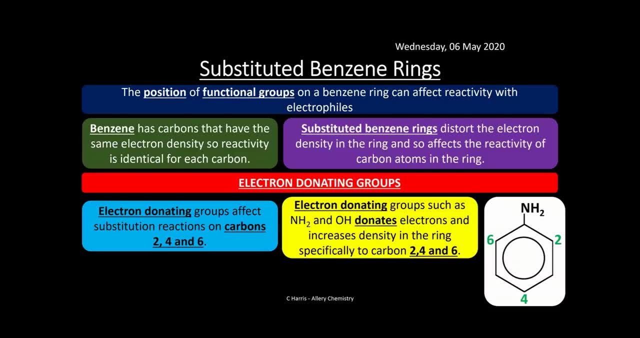 and six. but electron donating groups, such as nh2 and oh, donates electrons and increases the density of the ring, specifically at carbons three and five, because of the electron withdrawal nature of it. so therefore the electron is more likely to attack on carbons two, four and six, and so therefore, 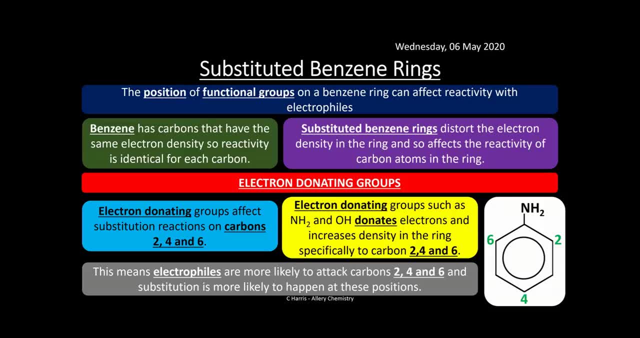 the electrophiles are more likely to attack on carbons two, four and six, and so therefore substitution is more likely to happen at these positions. so this is things like, for example, phenol, for example phenol reactions, um or phenyl amine, as is shown in that diagram there. 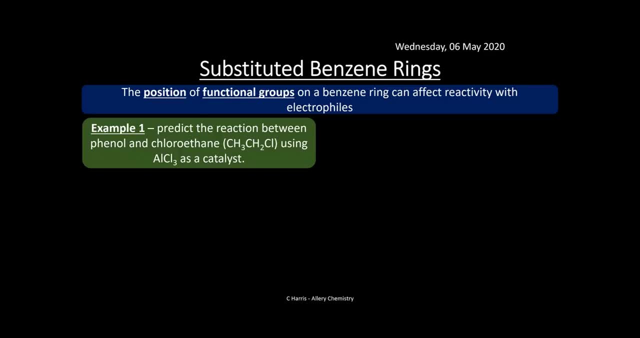 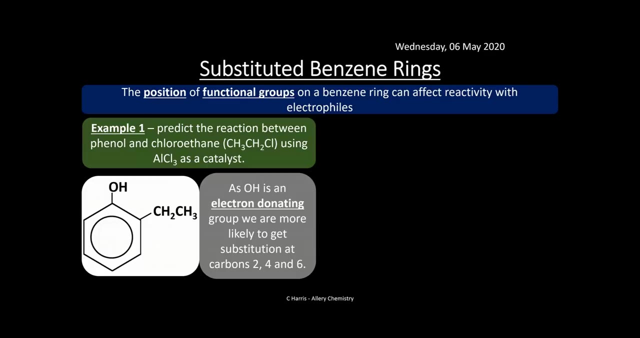 so let's look at an example of these different types of reactions. so let's predict the reaction between phenol and chloroethane, which is ch3, ch2, cl, using an alcl3 as a catalyst. so as the oh is an electron donating group, it pushes electrons into that, benzene into that. 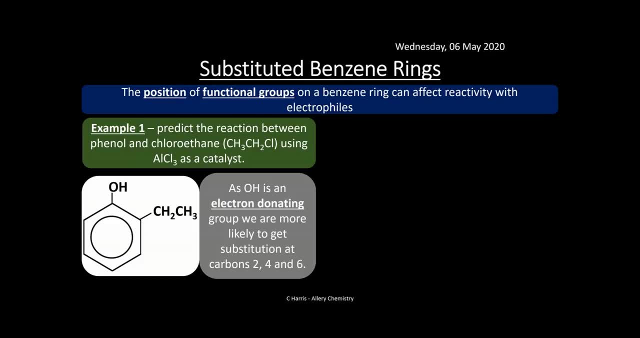 benzene ring structure, that delocalized structure, then we're more likely to get substitution at carbons two, four and six. now let's look at a second example. so predict the reaction between nitrobenzene and chloroethane. so here we've got a reaction between nitrobenzene and chloroethane. 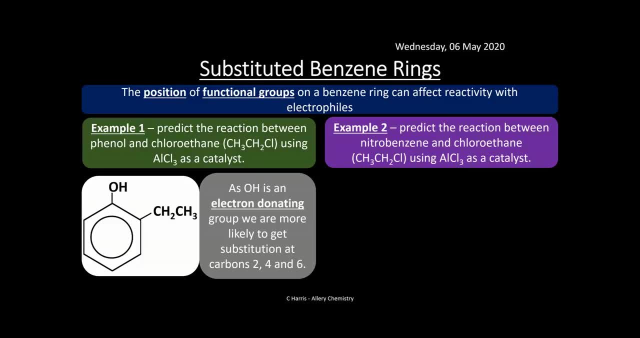 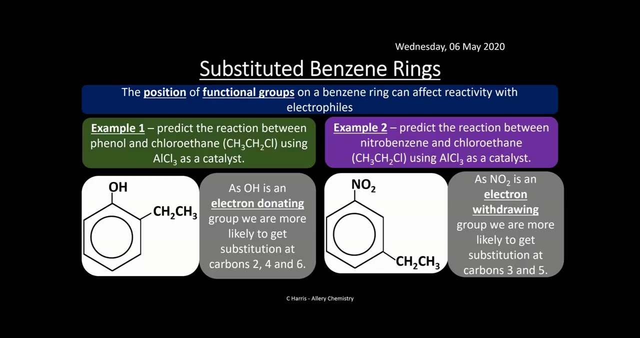 we've got a different type of um- um phenyl amine compound, we've got nitrobenzene um and we've got chloroethane, which is the same substance. so this time we've got an electron withdrawing group and so therefore we're likely to get substitution at carbons three and five. 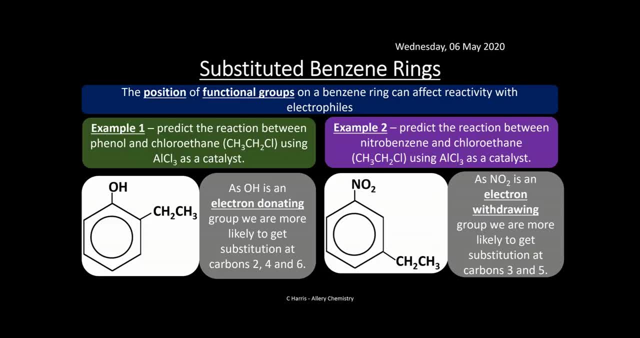 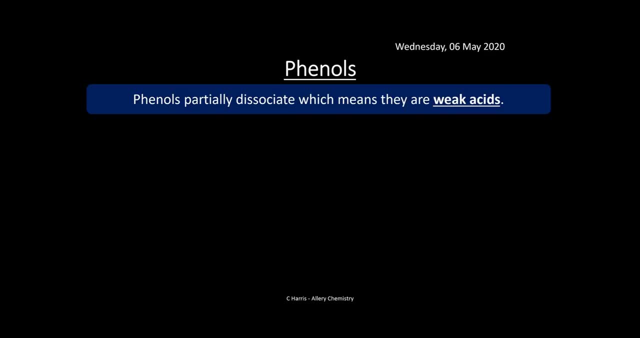 instead. so there's a stark difference. as you can see, it really does depend on what type of group, what type of reaction, whether it's going to be phenol or whether it's going to be um, say a nitro, a nitro- um compound. okay, so let's go back into phenols, in particular um and phenols partially dissociate, which means 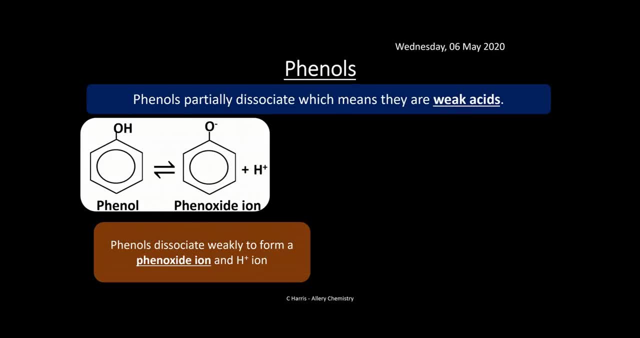 they're actually weak acids. so you can see here, here we've got phenol um and it's partially dissociating, losing its h plus. so remember, for something to be an acid, a bronzed larry acid, it loses its proton and therefore that's classed as an acid. but if it's a weak acid it means that equilibrium. 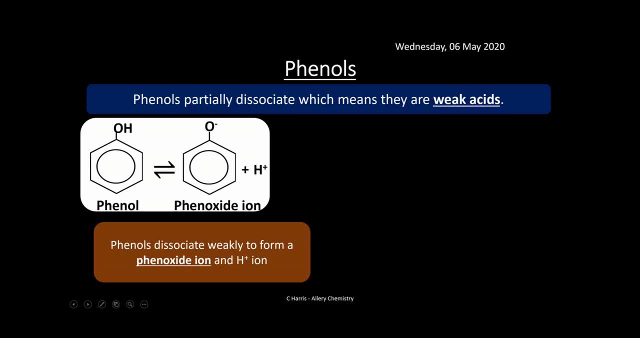 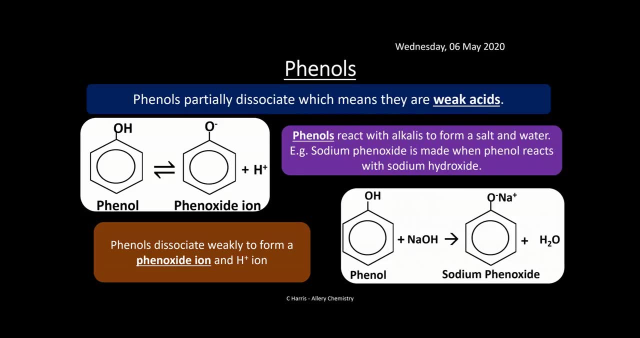 lies well over to the left, so you're going to get. it's not going to dissociate fully, so you're going to get a lot of this and not much of this. so phenols react with alkalis to form salt and water because they're an acid. they react in the same way as acid acid base reactions. so 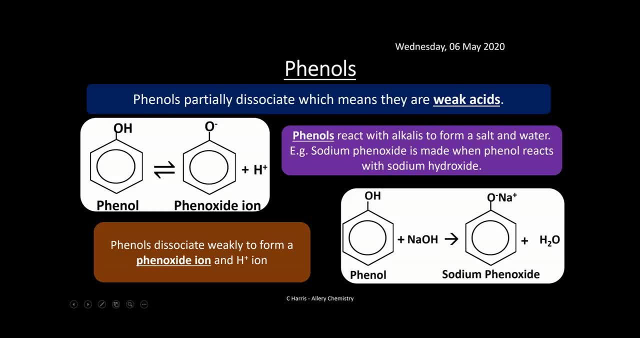 so this is going to form some salt and water. so in this case we're going to form sodium phenoxide. okay, so exactly the same as what you do with the saludimosaccharides acid base reaction, and we form water as well. so there's no difference there. it looks a little bit. 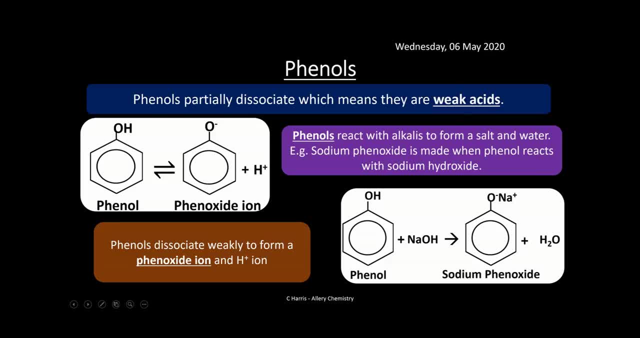 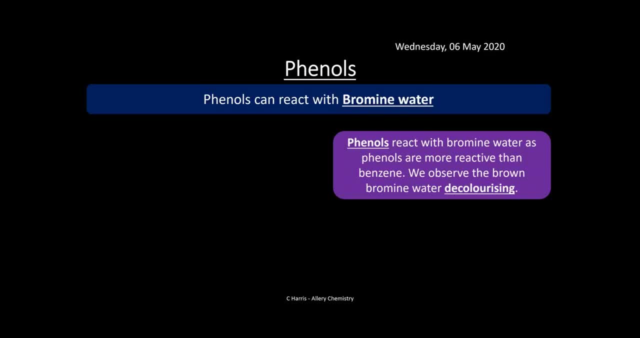 different because it's got a benzene ring stuck on it, um, but it's, it's um, it's a similar type of reaction, okay, so phenols can also react with bromine water as well. so phenols react with bromine water, um, as phenols are much more reactive than benzene, remember, because of that. 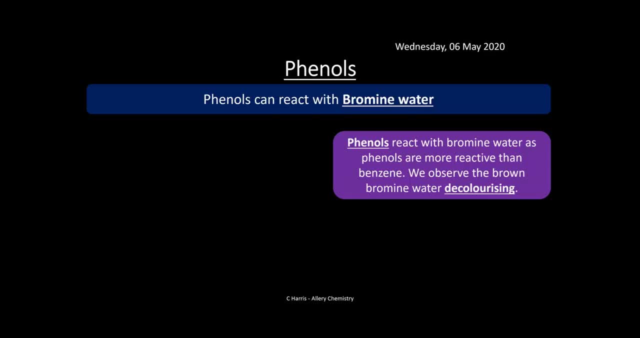 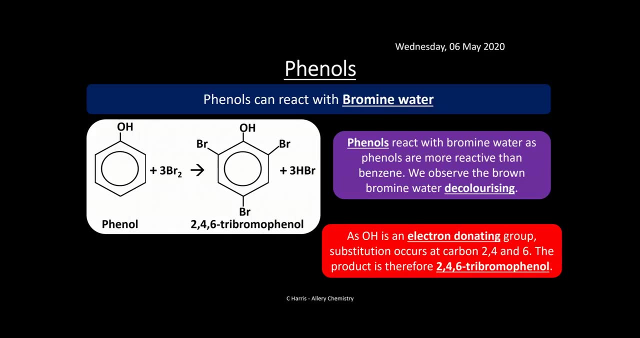 that ability to donate some of its electrons into that, into that um delocalized ring, and so what we observe is um decolorization of of bromine water. so you can see here, um, oh, is a an electron donating group, as we've said. so it pushes electrons into that, into that benzene ring. so the reactions 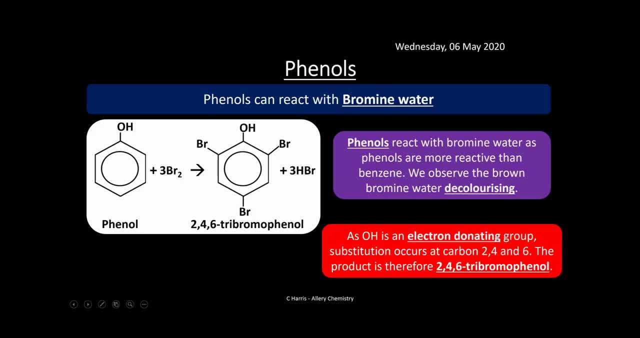 are more likely to happen at two, four and six. so we end up with a, with a compound which is two, four, six, tribromophenol, which we can see here, um, and also obviously we also produce three hbr as well, but we've decolorized it because we've gone from a brown 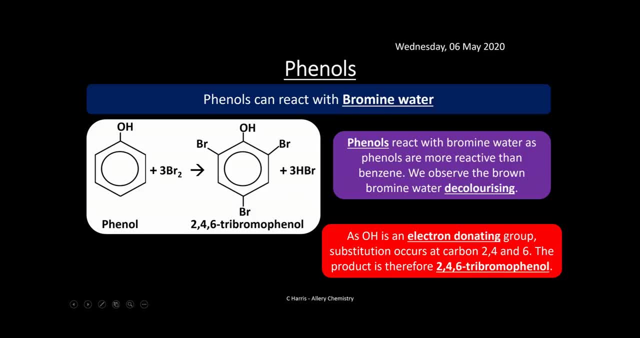 bromine to a decolorized um um tri-substituted uh phenol um. it smells of antiseptic, um, it's got this um. if you've ever had um a tcp before, which is trichlorophenol um instead of using bromine. 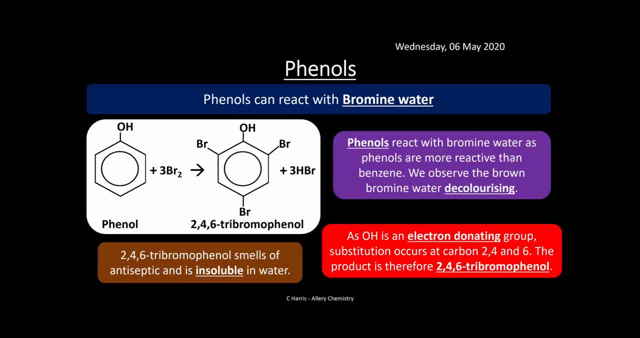 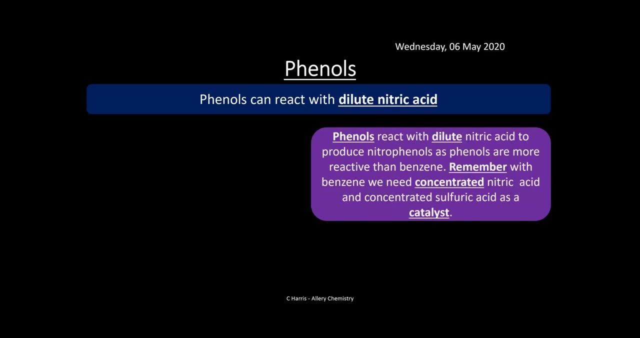 we use chlorine, um, then you'll know what it smells like. um, it's got that antiseptic smell, but, um, so it's very similar to that, and it is insoluble in water. so it's quite, uh, it's quite oily, okay, so phenols can also react with dilute nitric acid, um, and what they do is they produce nitrophenols. 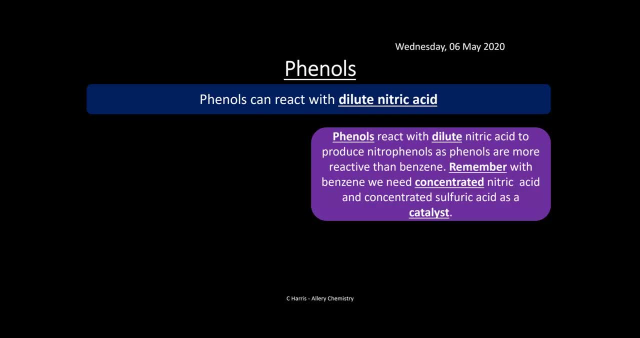 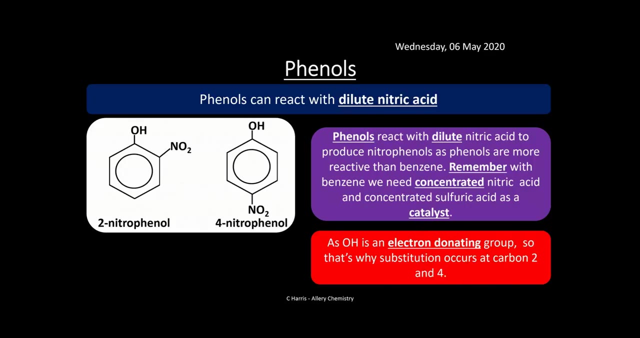 um, because phenols are much more reactive than benzene. so remember, when we tried to nitrate a benzene, we had to create um, a very strong, powerful electrophile. with phenols we don't need to, because they're much more reactive. um, so um, the oh is electron donating, so we get substitution. 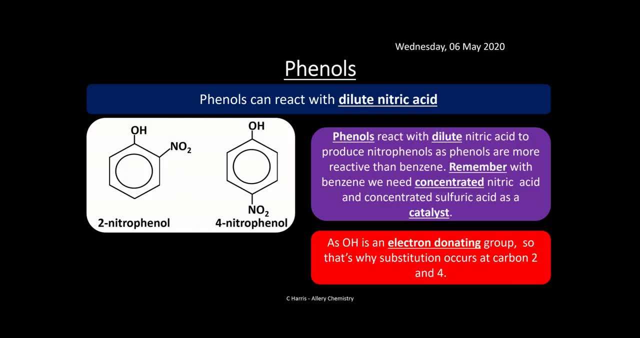 at carbons, two and four. so you can see here that we either get two nitrophenol or four nitrophenol. so this is the type of reactions that we get when we react phenol with dilute nitric acid. okay, so these are the two isomers that we can, that we can produce.